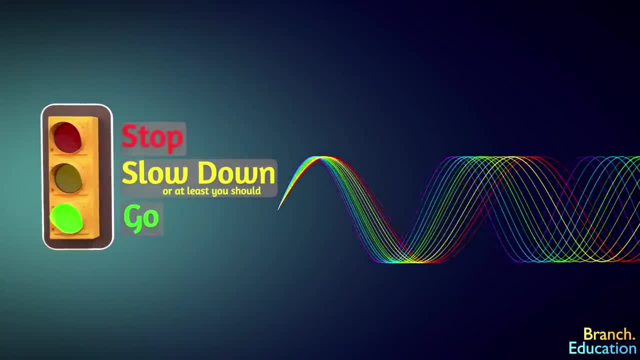 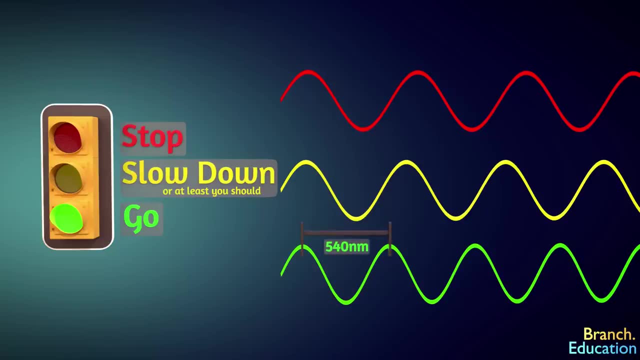 The traffic light uses a section of the electromagnetic spectrum or light to convey information. The green light has a wavelength of around 500.. Yellow around 540 nanometers, Yellow around 570 nanometers And red around 700 nanometers. 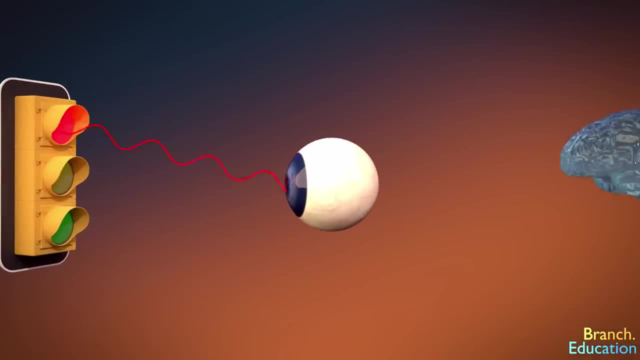 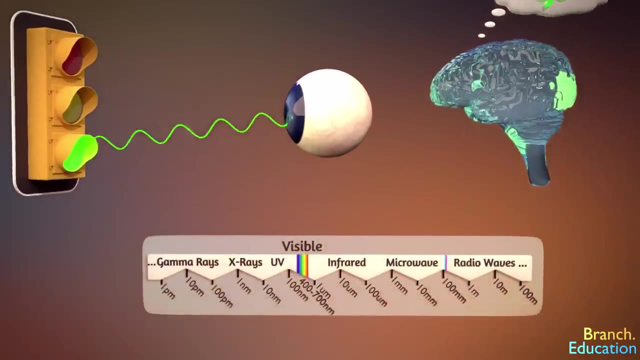 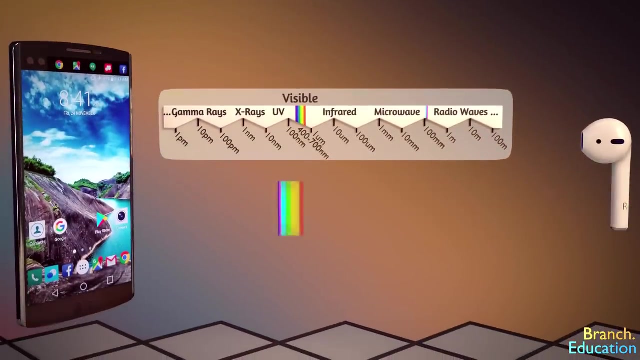 Your eyes can easily distinguish between these different wavelengths of light and your brain interprets these different wavelengths and the information they convey. Your smartphone and wireless earbuds communicate using electromagnetic waves in a rather similar fashion, but utilizing a different section of the spectrum. 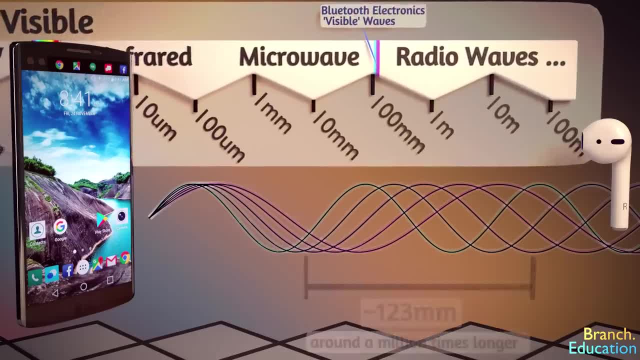 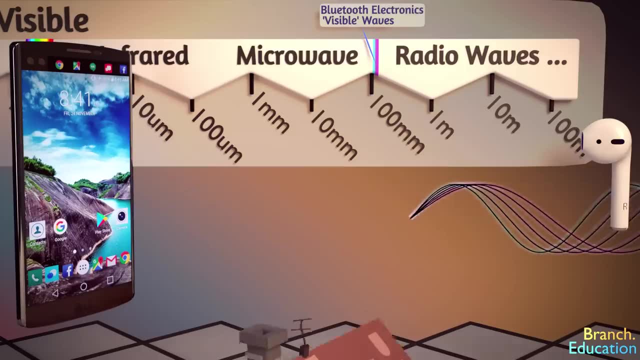 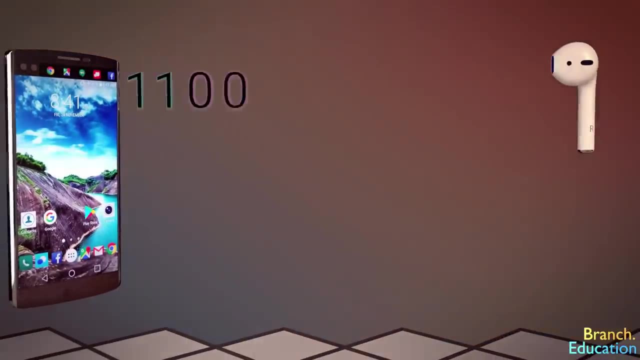 Specifically, Bluetooth uses waves that are around 123 mm in wavelength. They are invisible to the human eye and can generally pass through obstructions like walls, rather like visible light passing through glass. When your smartphone sends a long string of binary 1s and 0s to your earbuds, 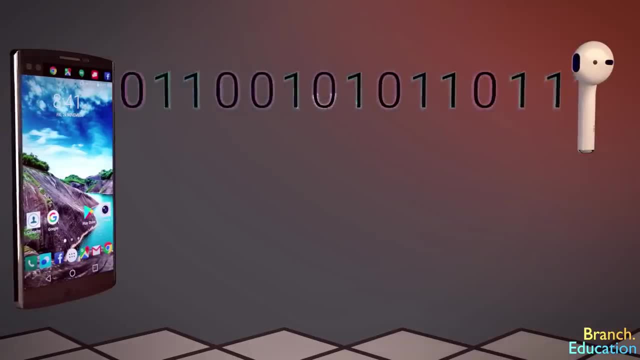 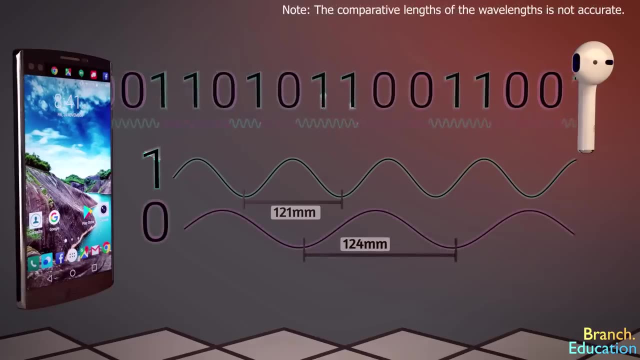 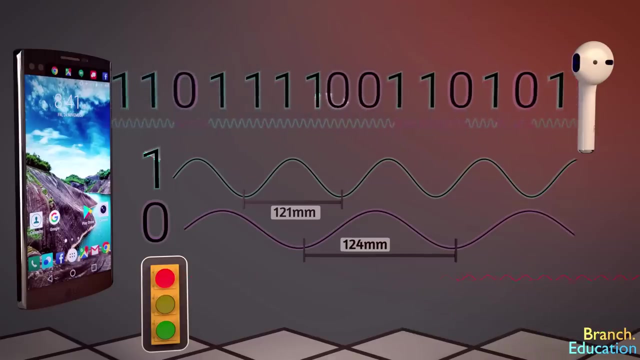 it communicates these 1s and 0s by designating a wavelength of 121 mm as a 1 and a wavelength of 124 mm as a 0, similar to the 540 nm green and the 700 nm red colors of the traffic light. 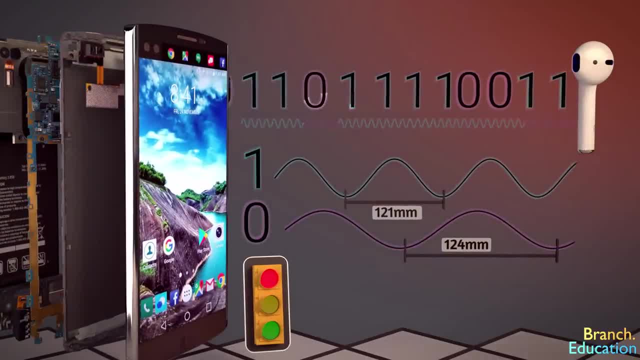 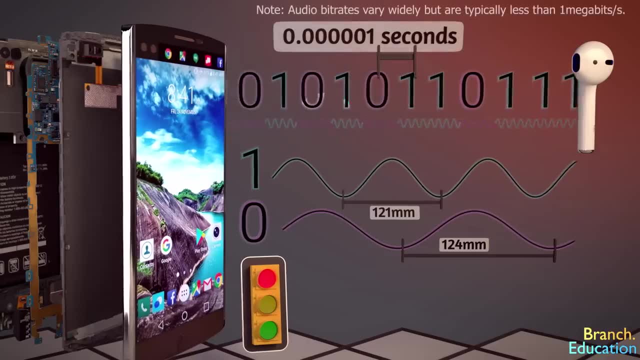 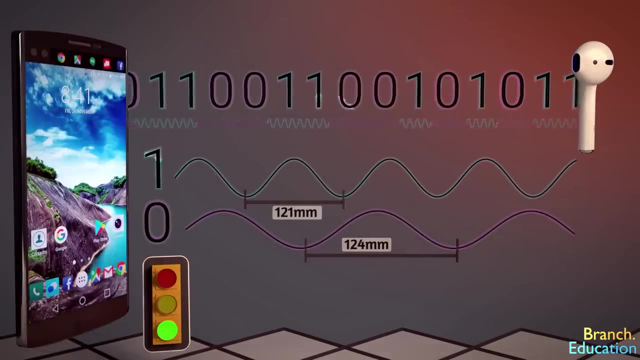 Your smartphone's antenna generates these two wavelengths and switches back and forth between them at an incredible rate of about a million times a second. With this process of switching between the two wavelengths, kind of like switching between the red and green traffic lights, your smartphone can communicate. 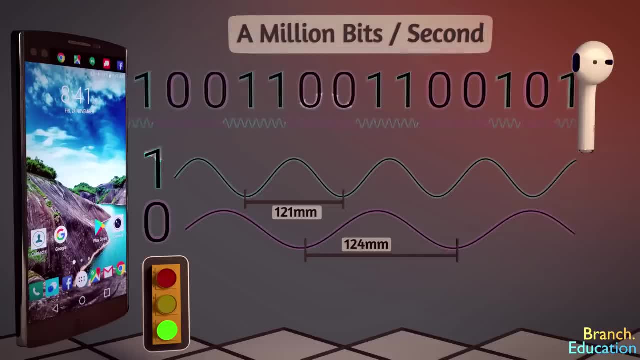 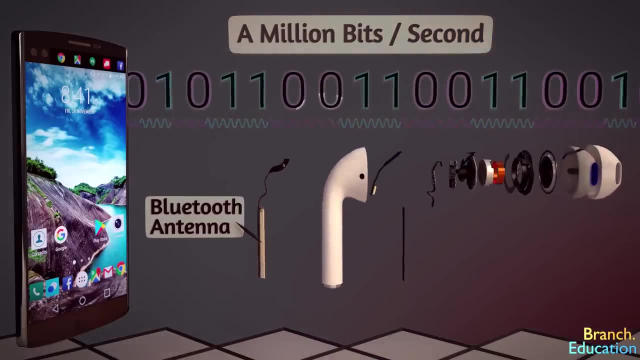 around a million 1s and 0s every single second to your earbuds And, amazingly, engineers have designed the antenna and circuitry in your earbuds and smartphone to be attuned to sensing and transmitting these wavelengths back and forth to one another. 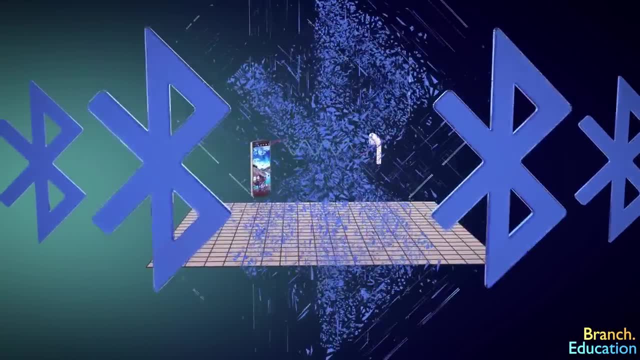 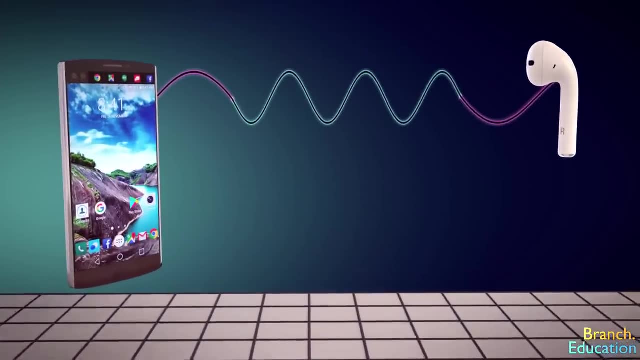 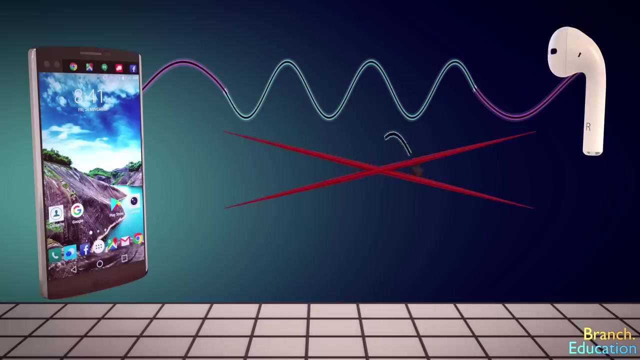 Before we dive into further details on Bluetooth, let's briefly explore and clarify these visualizations, because they're potentially rather confusing. First of all, electromagnetic waves do not travel in a single direction, in a sinusoidal fashion like this. In fact, the electromagnetic waves that are transmitted from your smartphone. 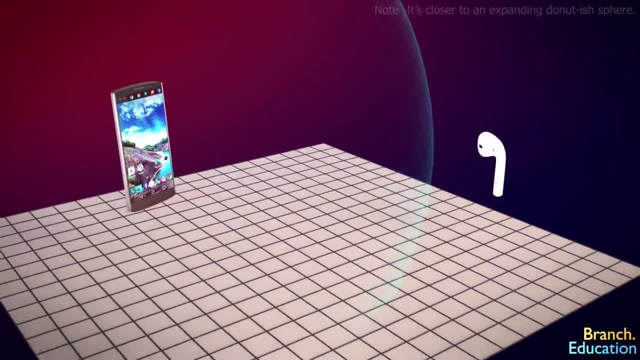 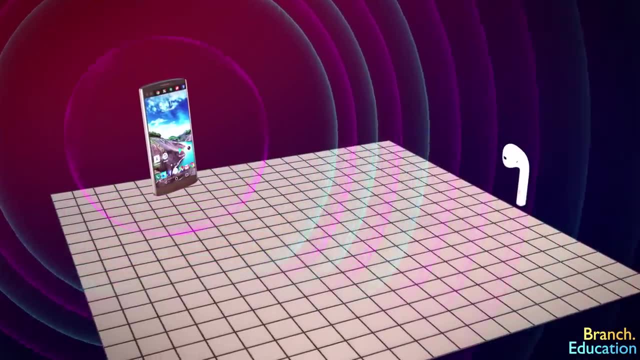 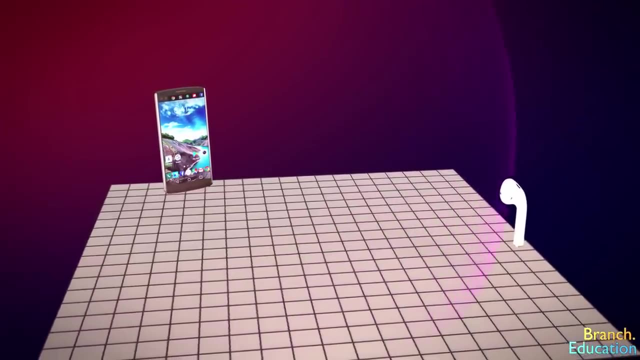 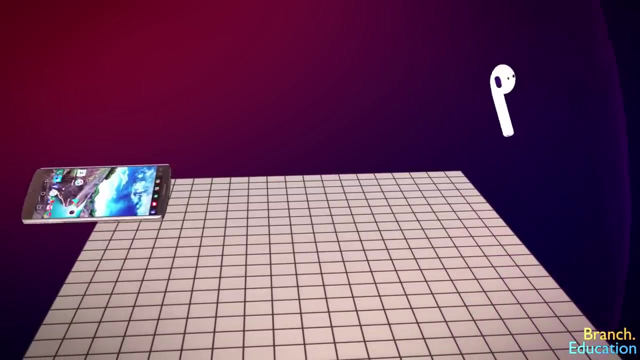 travel out in all directions like an expanding sphere. When your smartphone switches between frequencies, it's as if it were a light bulb that rapidly changes between two different frequencies of millimeter-length electromagnetic waves, which travel out as a constant. As a result, your smartphone and wireless headphones can work in any direction. 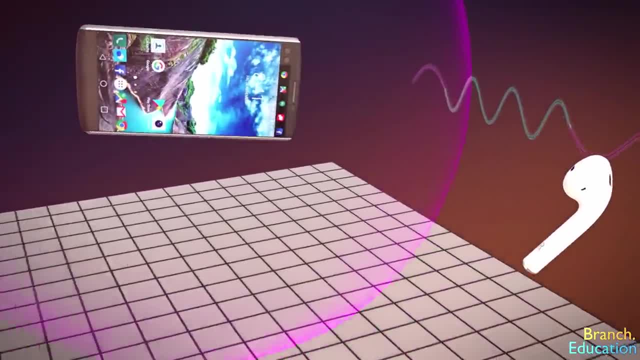 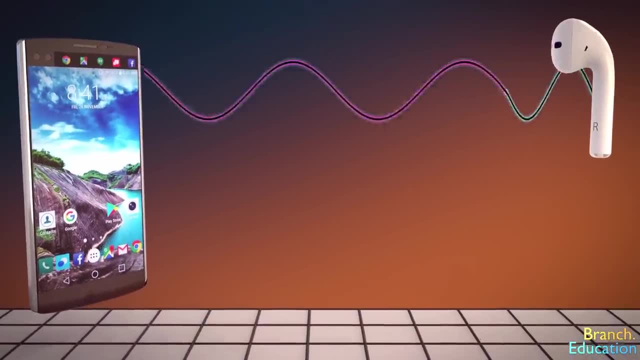 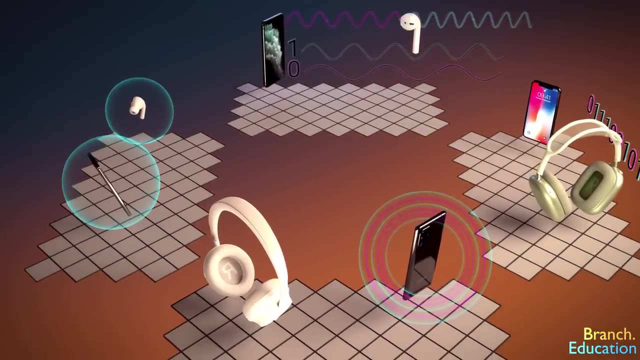 Thus, this visualization of a directional sinusoidal wave is lacking, Yet there are still merits to the visualization. In order to give you a sense of how Bluetooth works, we're going to use four different visualizations that are all different perspectives of looking at the same invisible thing. 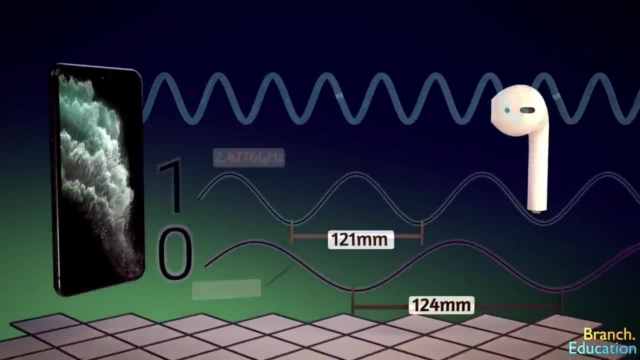 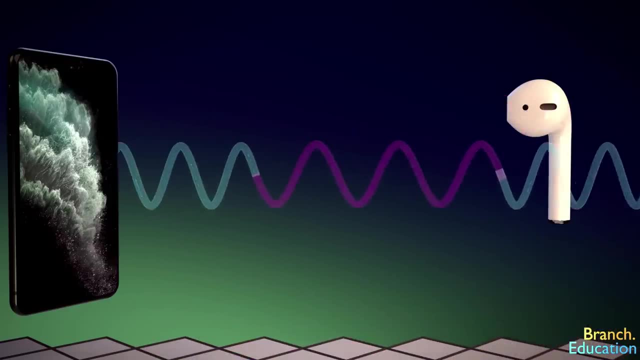 Here we have the sinusoid waves, which give us a sense of the frequency and wavelength of the electromagnetic wave. What's moving up and down is not the wave itself, but rather it's the strength of the electric field. This perspective just shows us a directional sliver or ray. 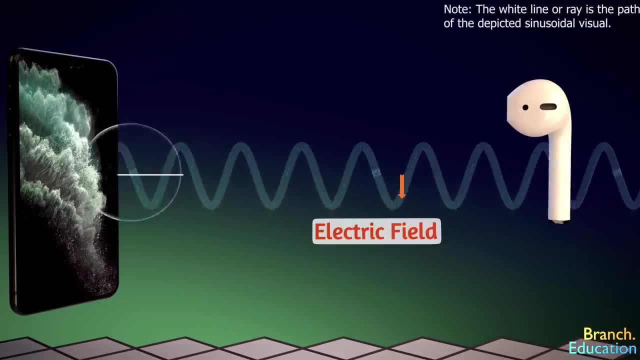 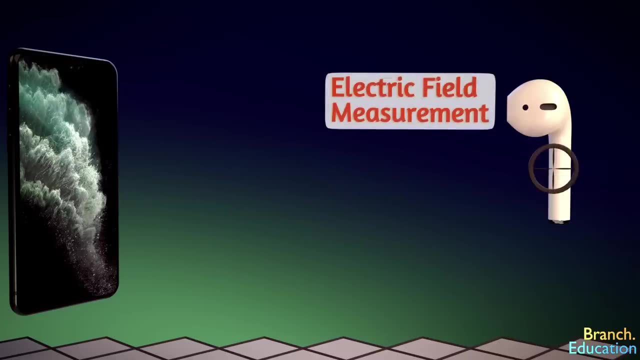 of the expanding sphere, with the electric field going up and down as the Bluetooth signal propagates outwards in all directions. If we were to measure the electric field at a single point or point in space, we would find that the strength of the electric field 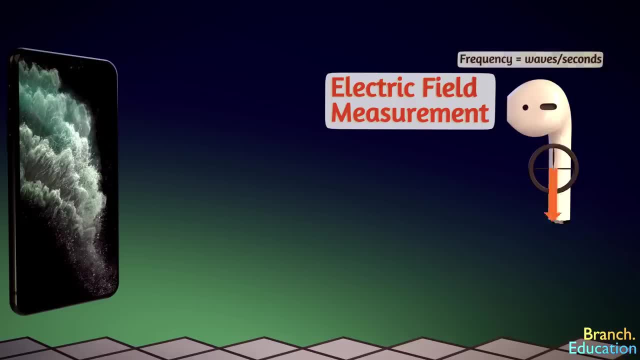 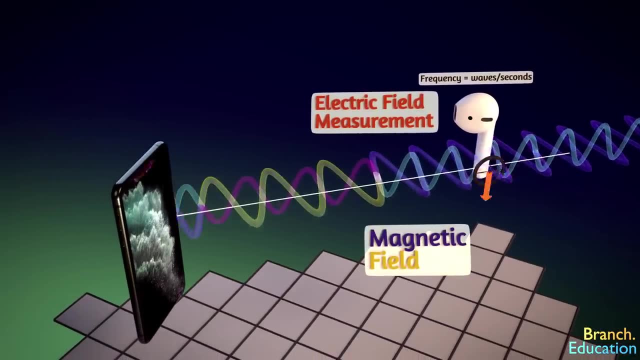 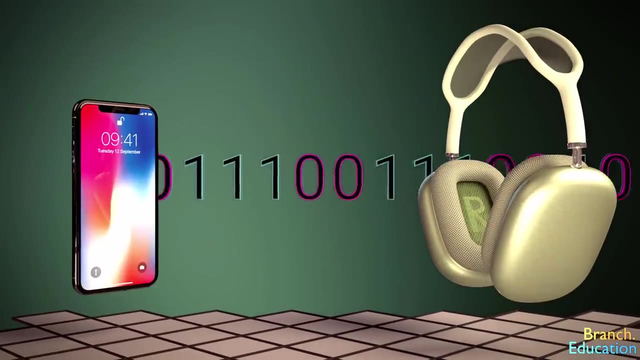 would increase and decrease sinusoidally and the number of peaks per second would be the frequency. Furthermore, we're ignoring the magnetic field component of the electromagnetic wave, as including it would be too confusing. Let's move on to the second visualization. 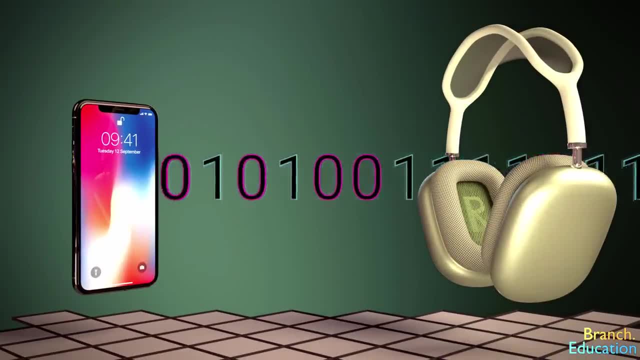 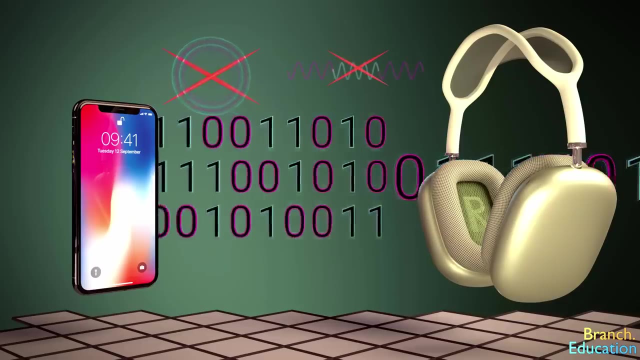 Here we have the traveling binary numbers, which give us a sense of the data being sent. However, it also doesn't show the spherical propagation of the electromagnetic waves or the changing frequency of the wave. Note that it's possible to send multiple bits at the same time. 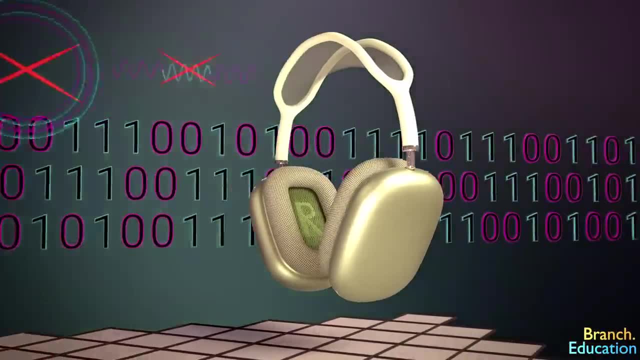 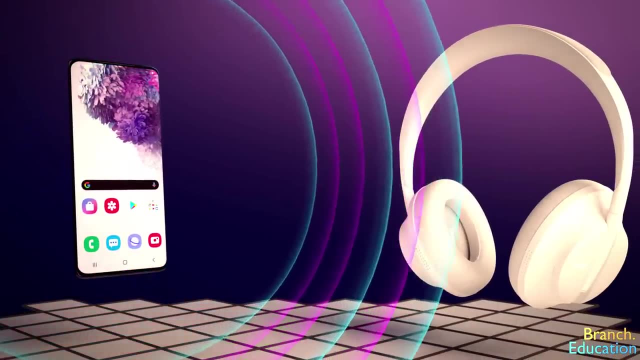 which we'll explore later. Third, we have the expanding spheres visualization, which gives a sense of the true, near omnidirectional emission of electromagnetic waves from your smartphone and headphones, But it's difficult to show the frequency or the data that's being sent. 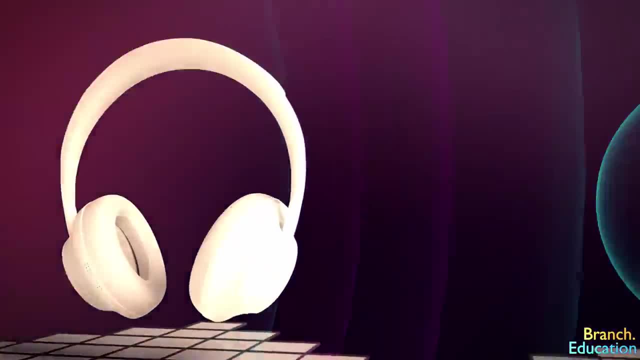 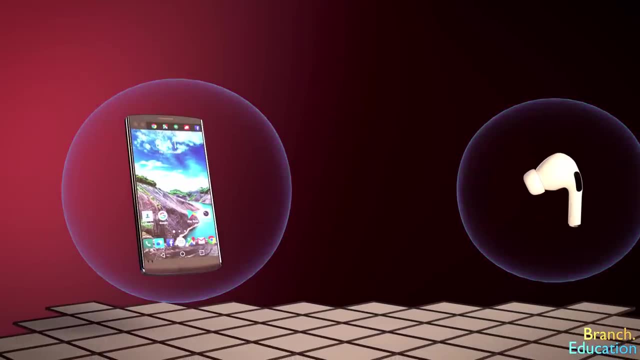 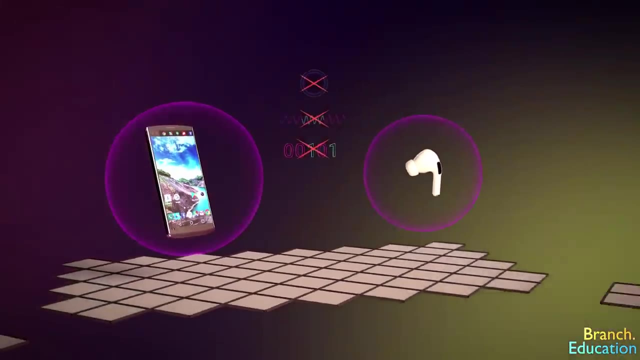 and it's rather visually complex to process. And last we have the simplified spheres which help us see that these two devices are emitting and receiving electromagnetic waves along the same frequencies, but it doesn't show us much else. Different visualizations are useful in different scenarios. 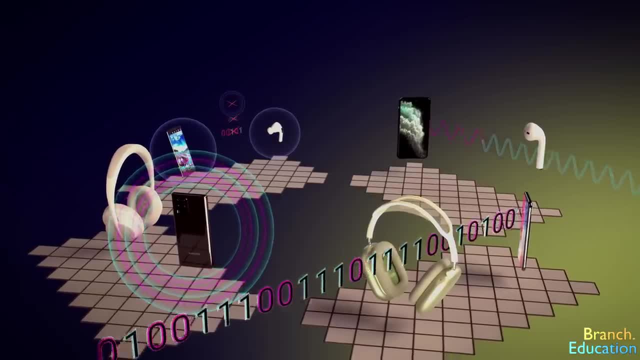 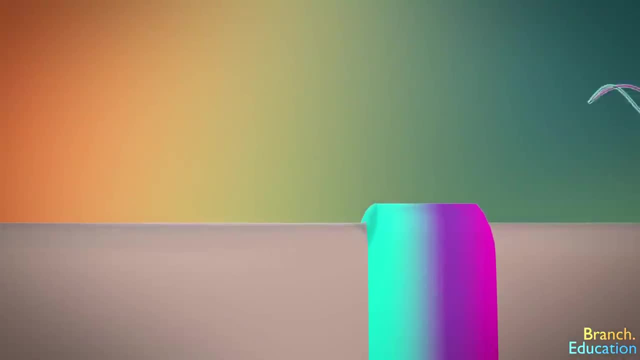 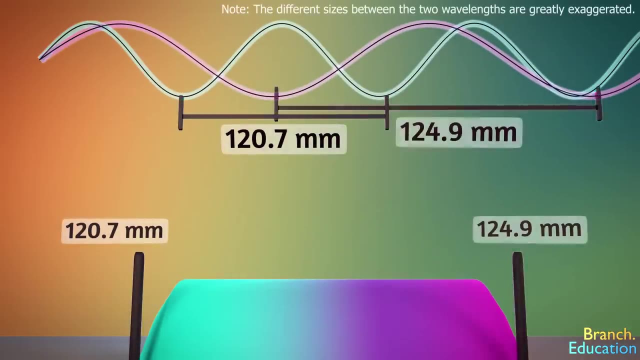 And with that covered, let's get back to the focus of this video. As mentioned, the electromagnetic spectrum operates at around 123 millimeters of wavelength, But specifically it operates between 120.7 millimeters and 124.9 millimeters of wavelength in the electromagnetic spectrum. Note that these frequencies are more commonly referred to as having a 2.4 to 2.4835 gigahertz frequency, bandwidth or range. Just as our eyes see within a range on the electromagnetic spectrum, Bluetooth antennas see or perceive within their own range of frequencies. 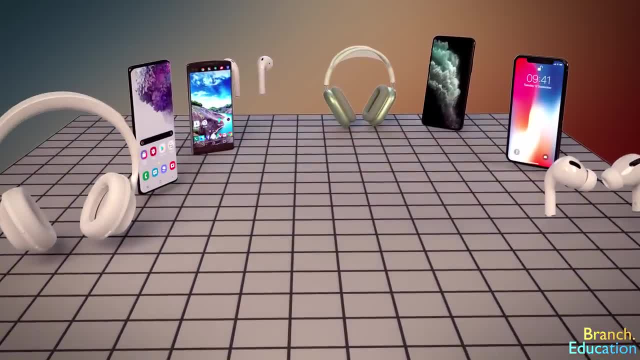 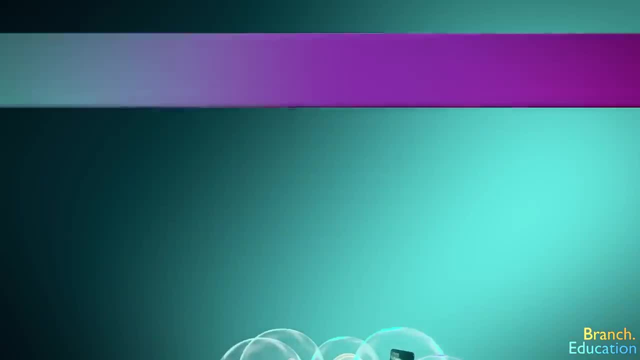 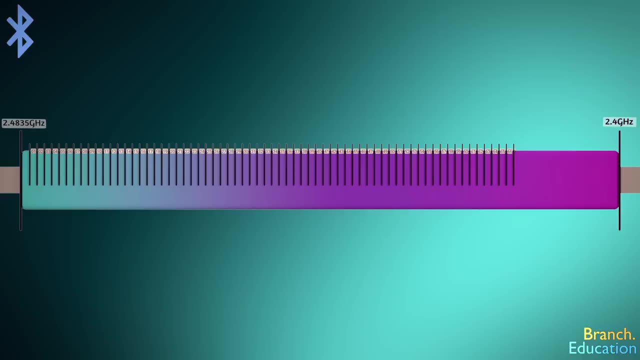 Now, at any given time, there might be dozens of people using Bluetooth devices at the same time in the same room. To accommodate so many users, this section of the electromagnetic spectrum is broken up into 79 different sections or channels, with each channel having a specific wave length. 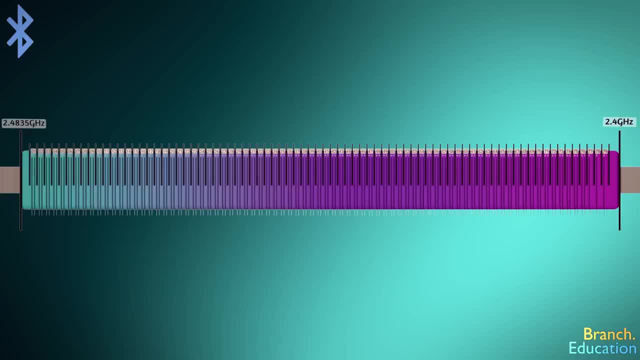 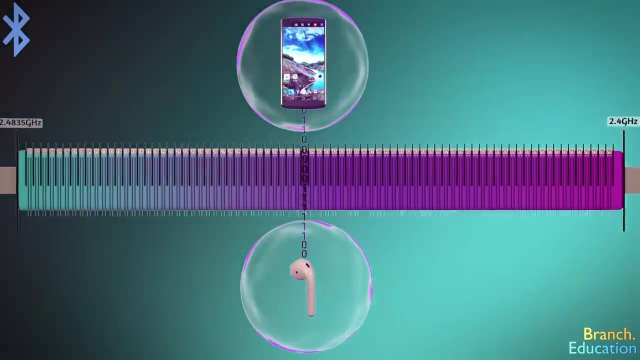 for a 1 and another for a 0. And at any given moment, your smartphone and earbuds communicate across just one of these channels. For example, these are the frequencies for a 1 and a 0 in channel 38,. 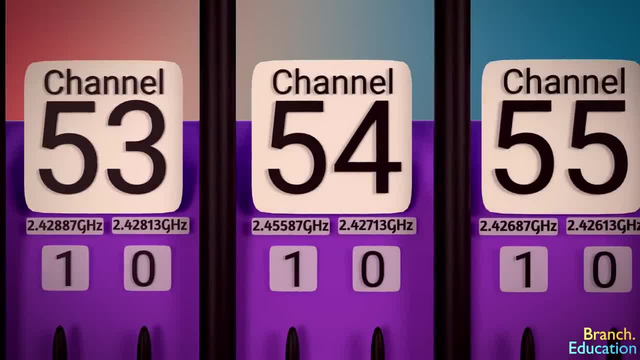 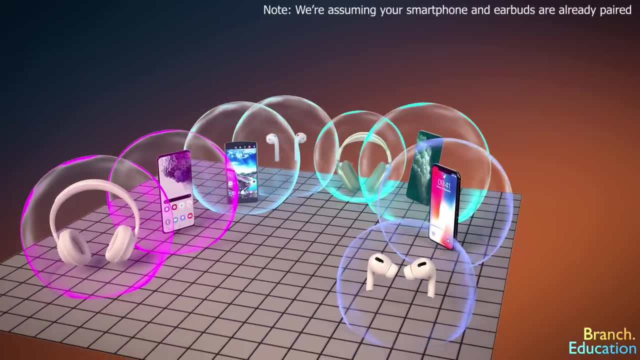 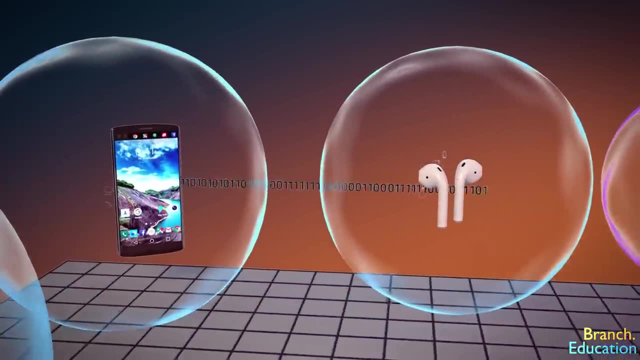 whereas these are the frequencies for channel 54. Now this begs the question: if dozens of devices are using the same wavelengths and possibly the same channel, how do your earbuds receive long, long strings of binary bits or messages from your phone exclusively? 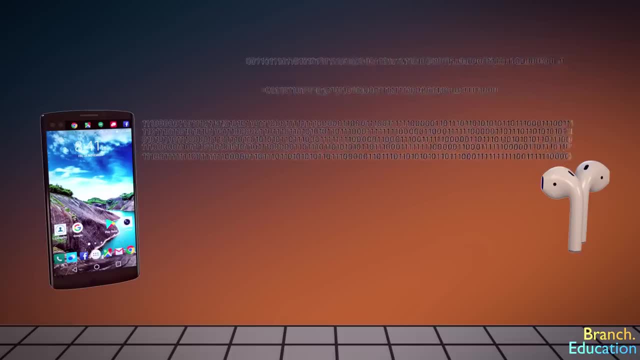 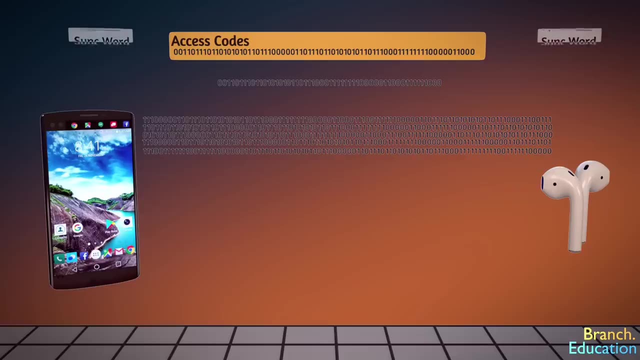 Well, first, the messages are assembled into packets. In each packet, the first 72 bits are the access codes that synchronize your smartphone and earbuds to make sure that it's your specific earbuds that receive the message. These access codes are similar to the address words. 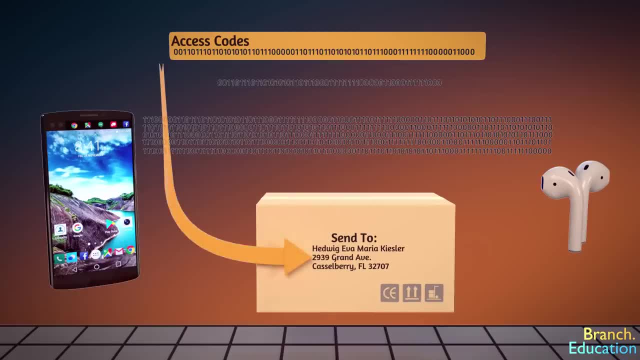 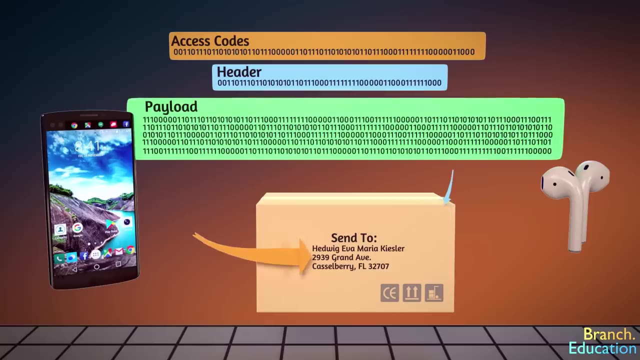 on a postal letter or package. The next 54 bits are the header, which provides details of the information being sent, which, in our analogy, can be equated to the size of the letter or the box, And the last 500 bits are the actual information or payload. 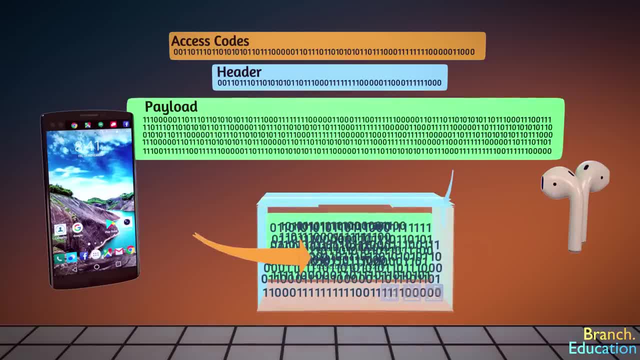 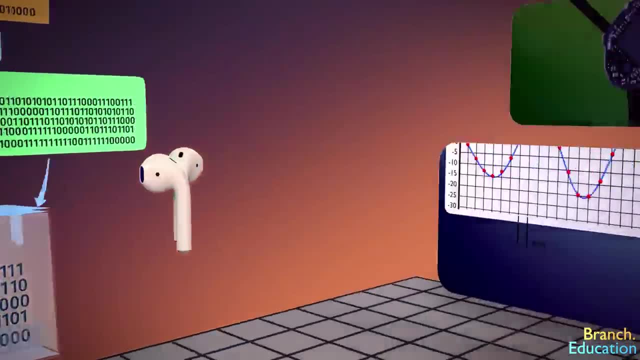 kind of like the contents of our postal letter or box, which in this case are the digital 1s and 0s that make up the audio that you're listening to. If you're wondering how audio can be represented by 1s and 0s, 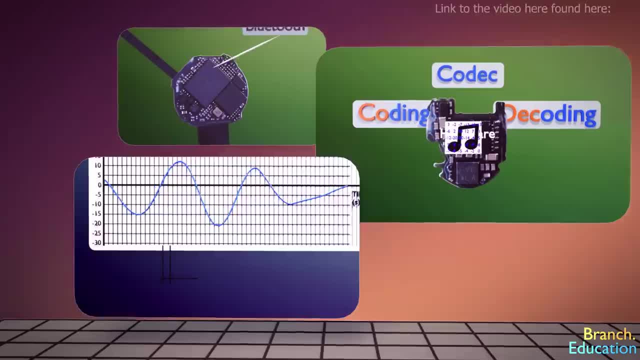 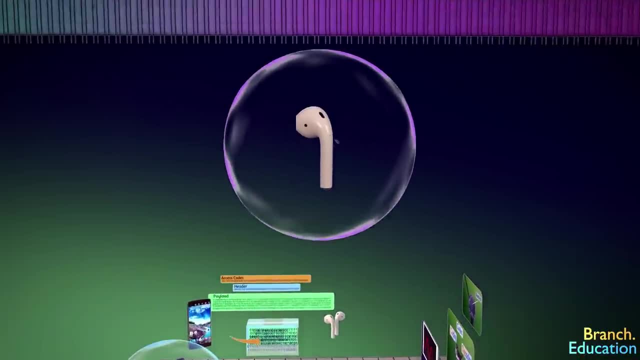 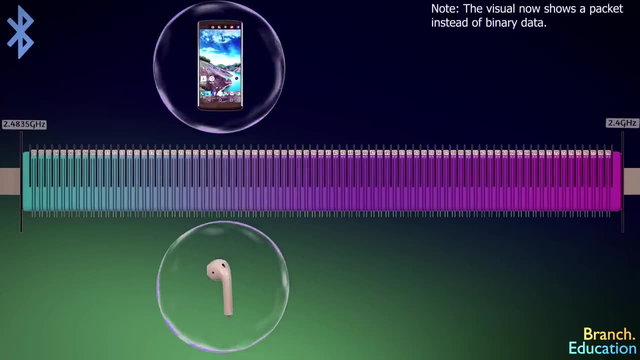 take a look at this episode on audio codecs. Okay, so now let's add more complexity to the mix. As mentioned, Bluetooth operates in a set of 79 different channels. However, when your smartphone and earbuds communicate, they don't stick to a single channel. 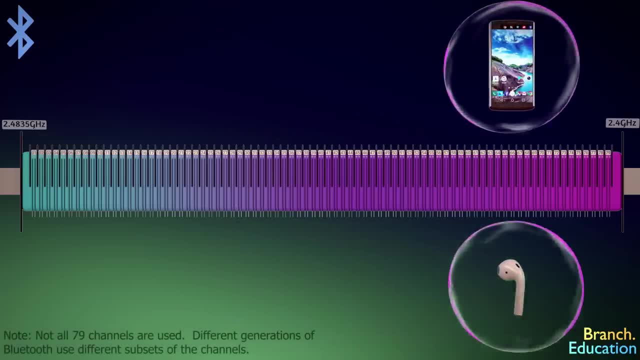 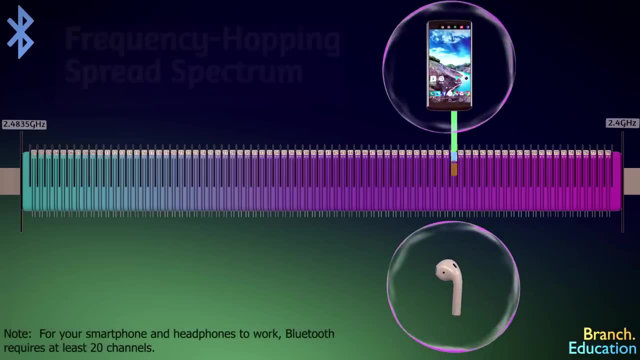 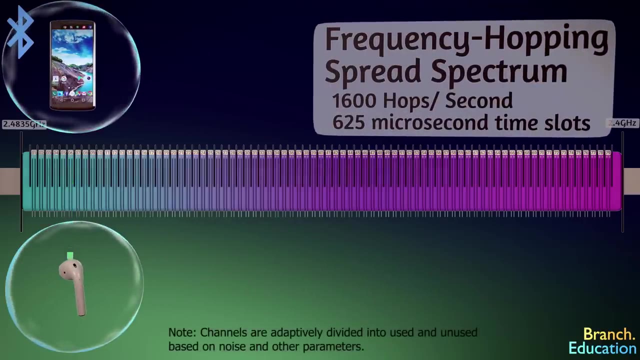 but rather they hop around from channel to channel, kind of like channel surfing on your TV. In fact, this hopping between the 79 channels, which is called frequency hopping, spread spectrum, happens 1,600 times a second, And after each hop, one packet of information. 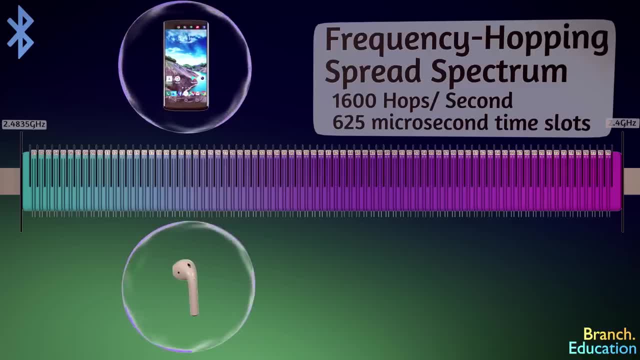 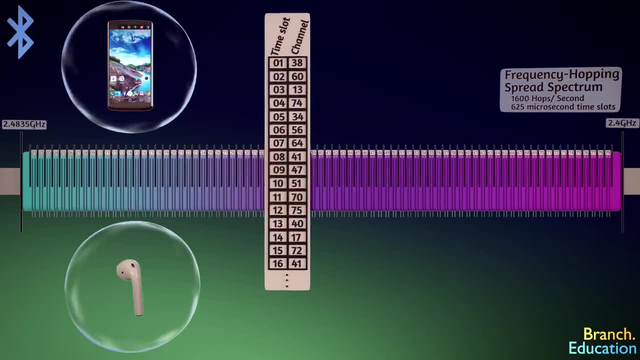 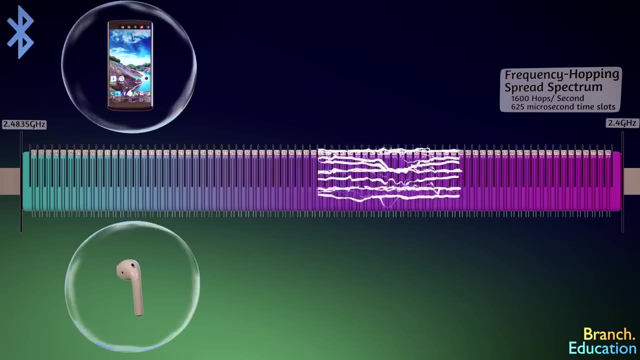 composed of the address header and payload, is sent between your smartphone and earbuds. Your smartphone dictates the sequences of channels it will hop to and your earbuds follow along. Furthermore, if one of the 79 channels is noisy due to interference, 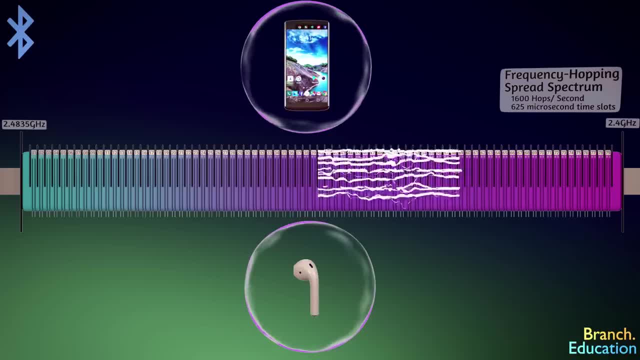 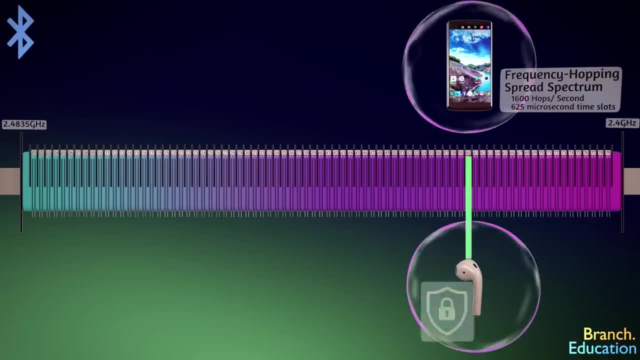 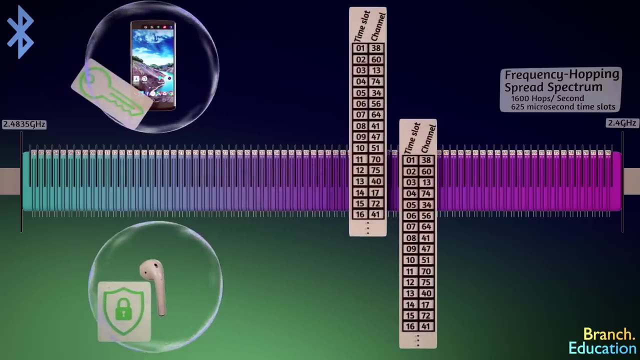 or is crowded with other users, then your smartphone adapts and doesn't use that channel until the noise clears. This channel hopping also prevents anyone from eavesdropping on the information that's being sent between the two devices, because only your smartphone and earbuds know the sequence of channels. 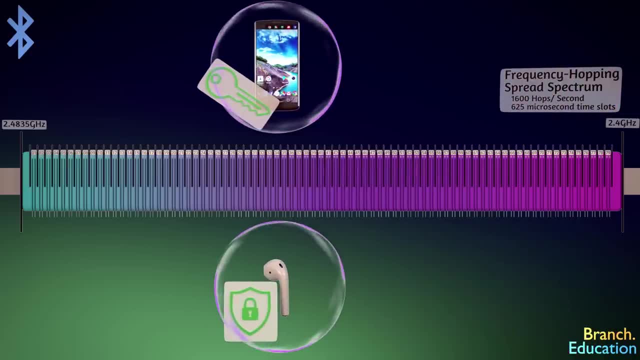 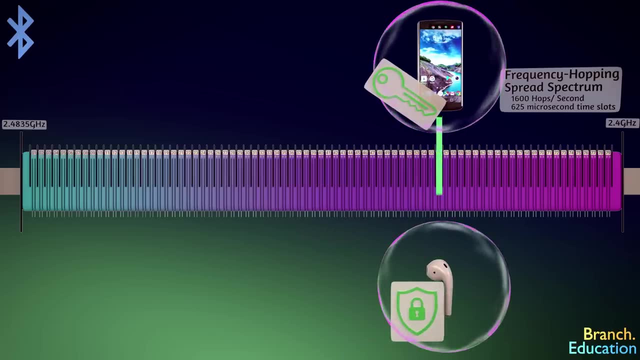 that they will communicate across. Interestingly, because the information is divided and sent using packets. if your earbuds don't receive one of the thousands of packets, it says it didn't receive it. It says it didn't receive that particular one. 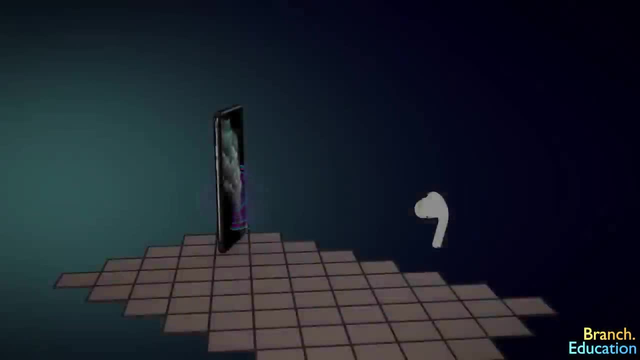 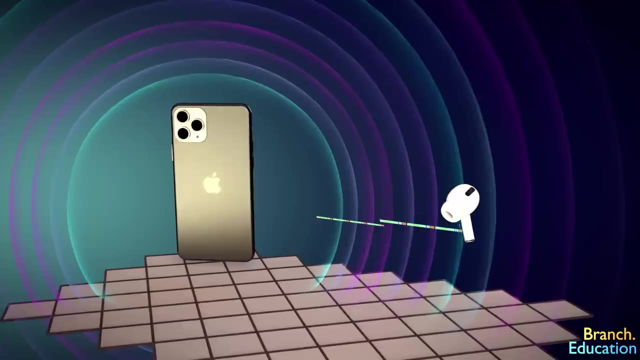 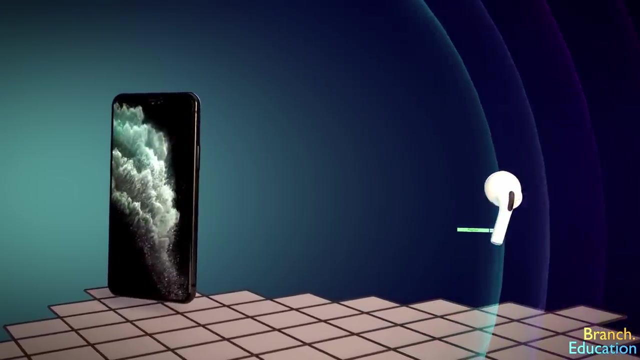 and your smartphone sends the packet again. It might seem crazy or mind-blowing that the circuitry in your phone can generate pulses of electromagnetic waves a million times a second at very specific frequencies, and then have these pulses received and decoded by your earbuds. 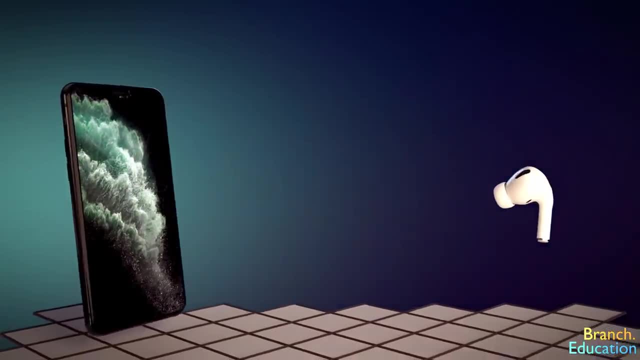 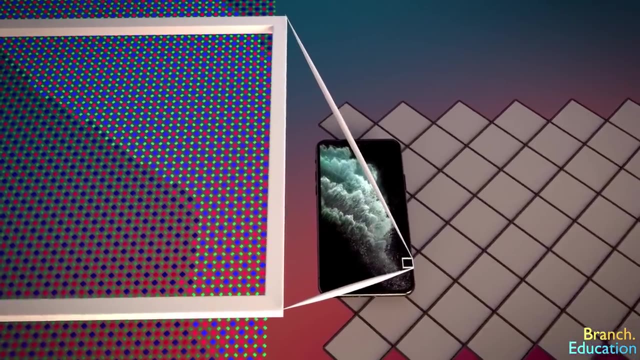 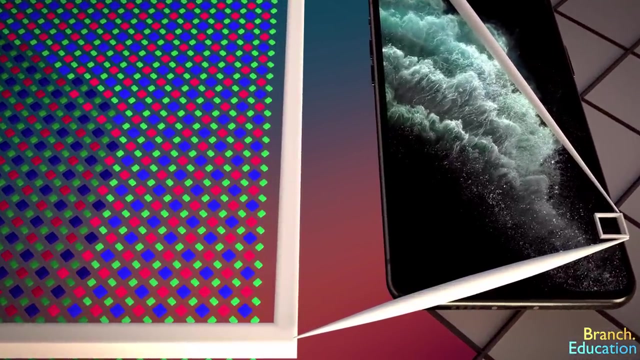 But hey, it happens. Just think about how your screen has millions of pixels also emitting specific frequencies and strengths of the electromagnetic spectrum or light at around 30 to 60 or more times a second. Technology is fascinating. One quick side note. 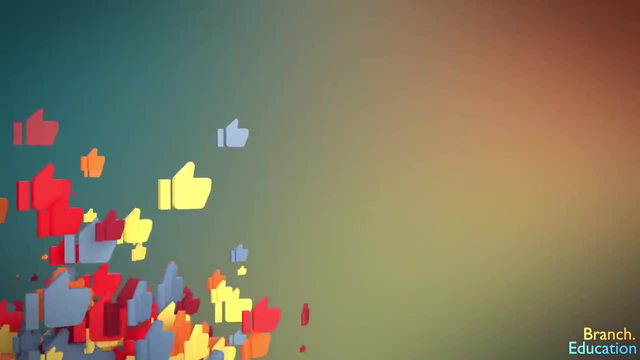 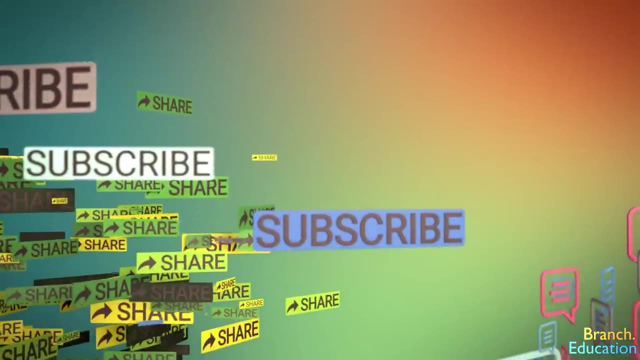 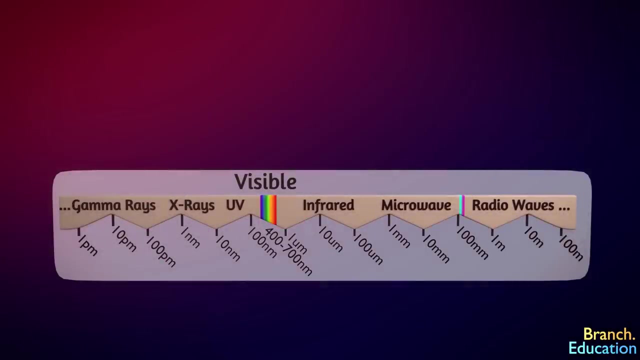 We would greatly appreciate it if you could take a second to like this video, subscribe to the channel, comment below and share this video with others. A few seconds of your time can help us to create many more educational videos. Thank you, Okay, let's move on. One point of interest is that Bluetooth's frequency range of 2.4 GHz to 2.4835 GHz is shared by other industrial and medical devices. For example, your microwave is in this range and has a frequency of 2.45 GHz. 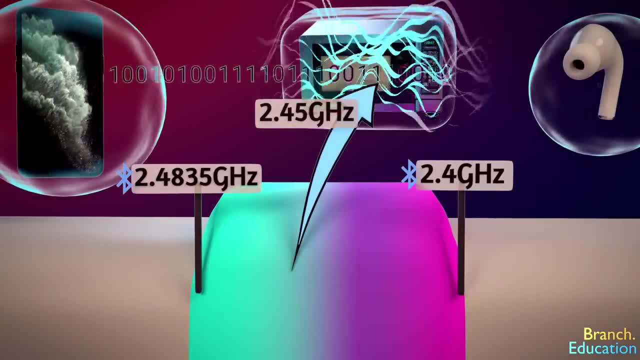 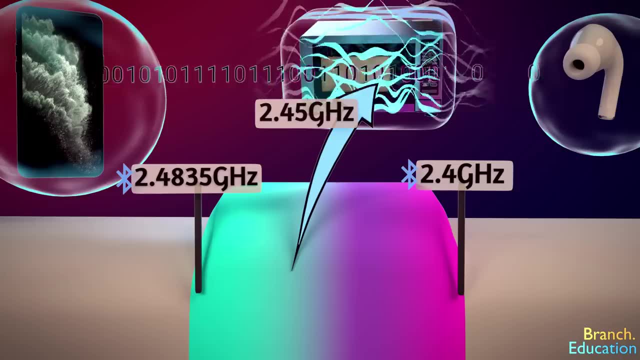 In fact, when your microwave is on, it can cause your headphones to lose track of the ones and zeros being sent by your smartphone, Or in other words, your headphones can lose signal. However, please don't think your Bluetooth headphones are dangerous. 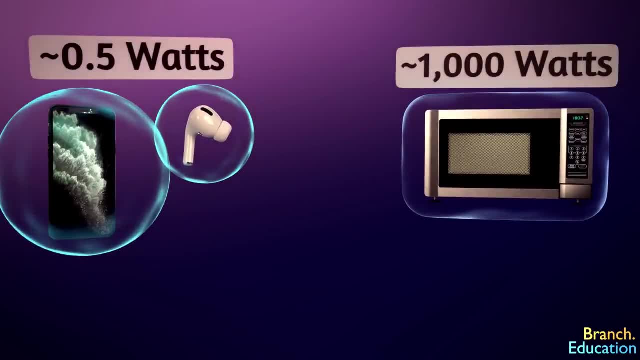 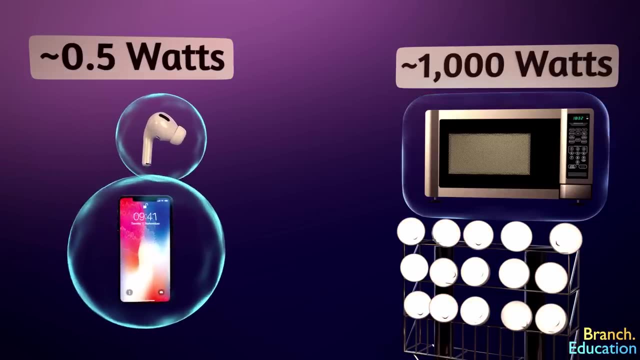 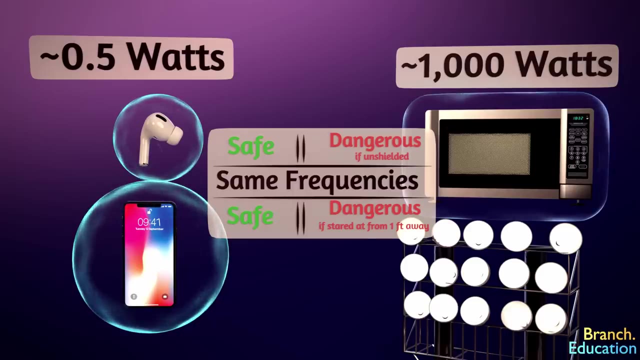 because they emit a wavelength that's similar to your microwaves. That would be like comparing the light output from stadium floodlights to the light from your smartphone's screen and saying that because they both use the same colors of light, they'll both cause damage when stared at from a foot away. 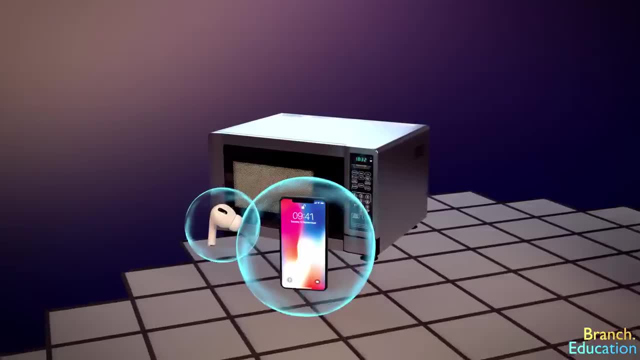 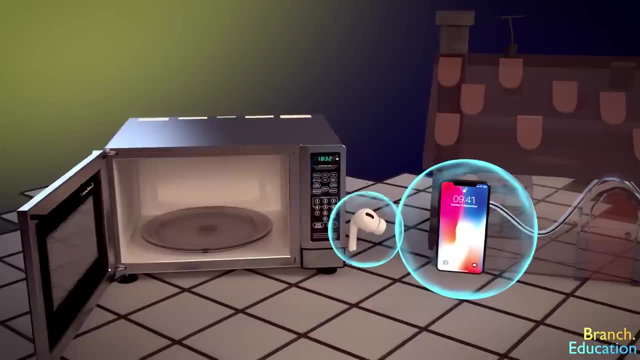 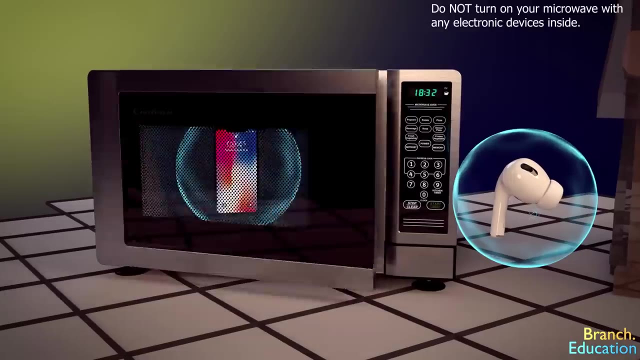 Also remember we mentioned that the electromagnetic waves from Bluetooth can easily travel through obstacles such as the walls of your house. However, the walls of the microwave are designed to block waves of this frequency. You can test this by putting your smartphone in the microwave. 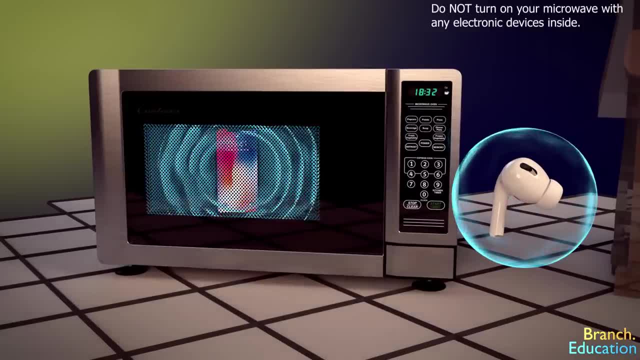 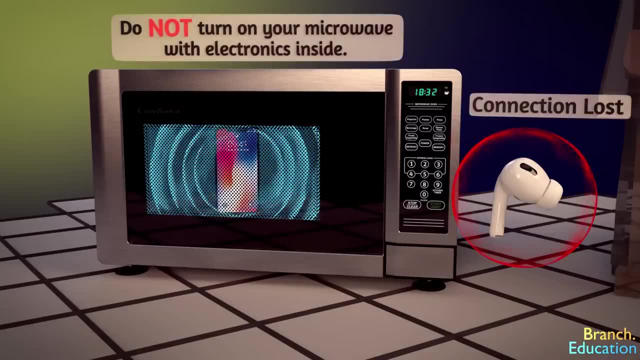 The Bluetooth signal from your smartphone to your headphones will be blocked and the connection lost. However, make sure not to turn on your microwave with any electronic devices inside of it. I repeat: do not turn on your microwave, otherwise it will damage whatever electronics you put into it. In addition to microwave ovens, 2.4 GHz Wi-Fi networks also operate within this range of the electromagnetic spectrum. Similar to Bluetooth, Wi-Fi networks divide this range or bandwidth into 14 channels in order to accommodate multiple users communicating via Wi-Fi at the same time. 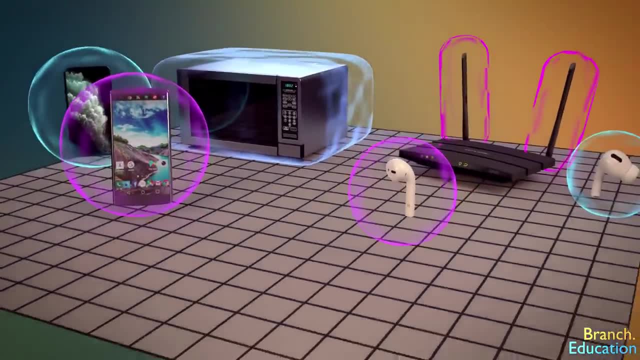 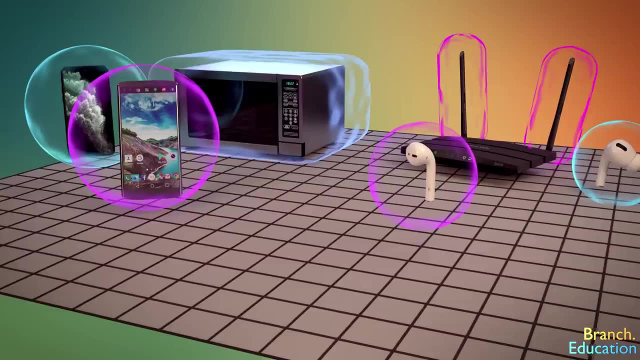 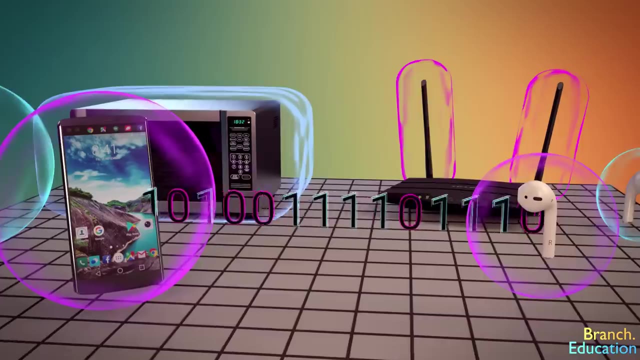 You might be wondering if there are a bunch of different devices all sharing similar frequencies, one of them being a microwave that, if poorly shielded, can emit stray electromagnetic waves. how is it possible for your smartphone and headphones to send megabits of data? 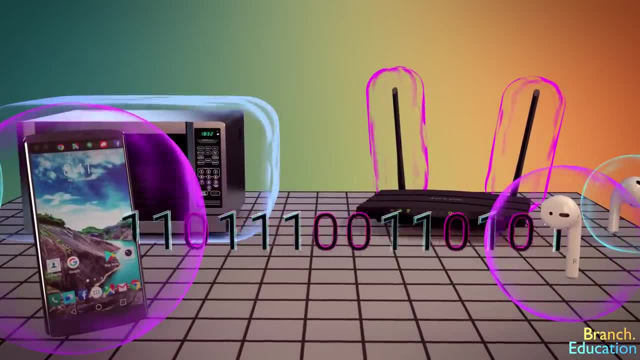 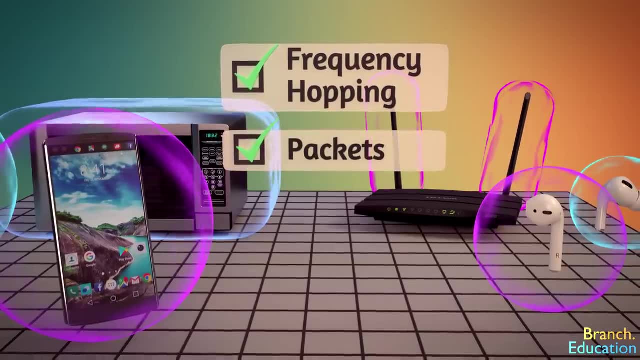 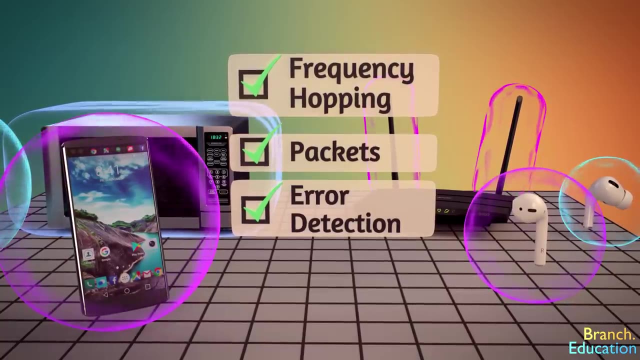 every second error-free. Well, as mentioned earlier, your smartphone does this by frequency hopping and utilizing packets. In addition to that, Bluetooth also utilizes bits for detecting errors, and the circuitry in your smartphone filters out unwanted noise. For a non-technical understanding of this: 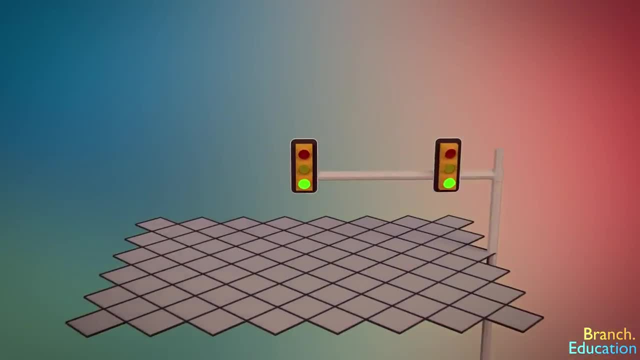 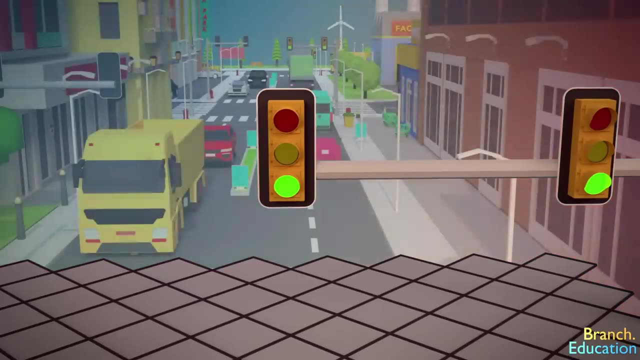 let's go back to our traffic light analogy. When you're driving and you see a traffic light, it's not like that's the only thing you can see. Your eyes perceive a rather complex scene filled with tons of other objects. Your brain interprets this information. 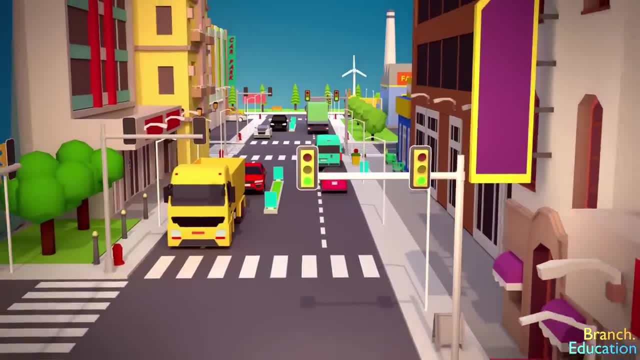 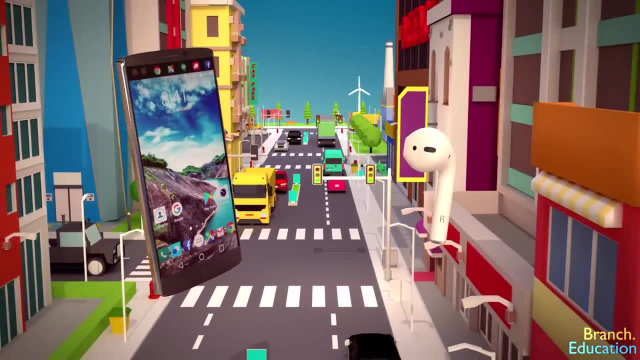 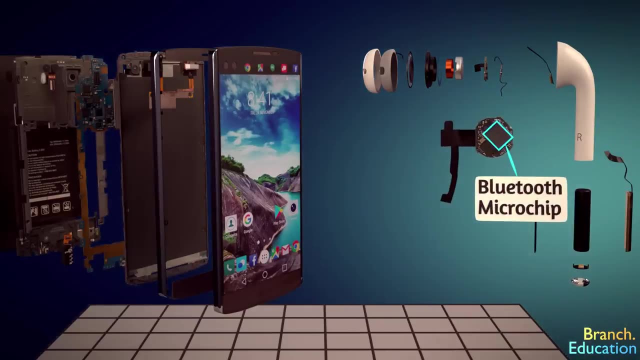 filled scene and picks out the information important to you while ignoring all the objects that aren't. Similarly, your smartphone and wireless headphones have rather complicated circuitry inside a specialized Bluetooth microchip that's designed and tested by engineers, which filters out unwanted signals. 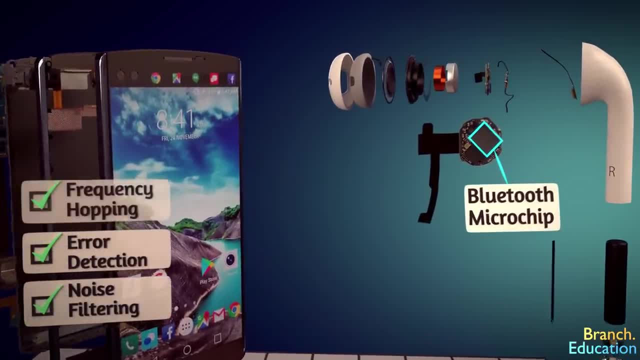 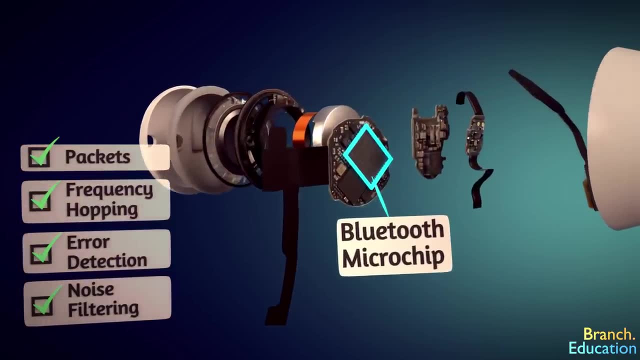 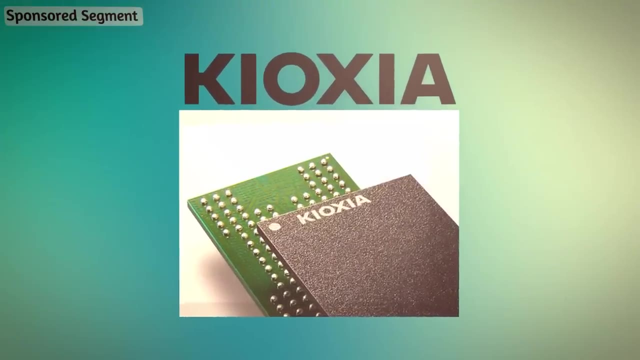 checks for errors, coordinates the frequency hopping and assembles the information into packets, thereby enabling reliance on reliable and secure communication. Before we move on to some higher-level engineering concepts, we'd like to take a few seconds to thank Kioxia for sponsoring this video. 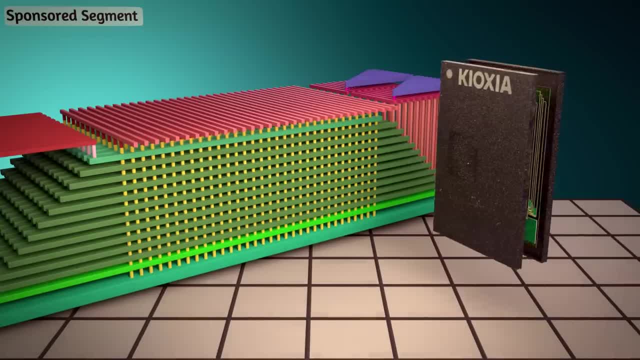 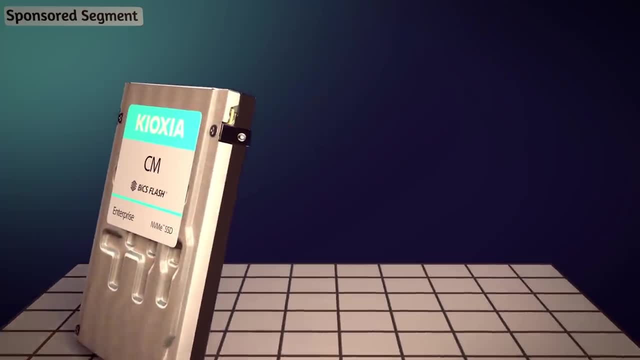 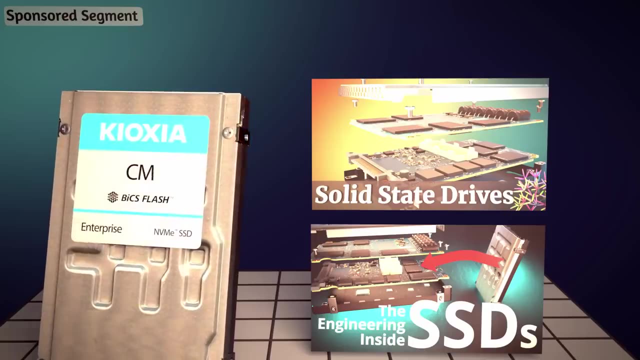 Many Bluetooth devices, such as mobile phones and tablets, use Kioxia Bix flash memory. Kioxia also manufactures a wide variety of SSDs, and they have sponsored a couple of our videos that explore the inner workings behind how SSDs work. 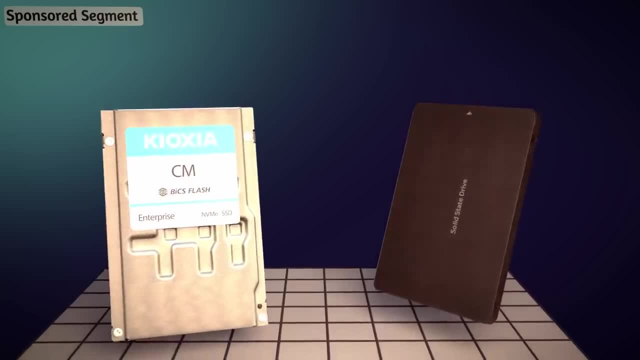 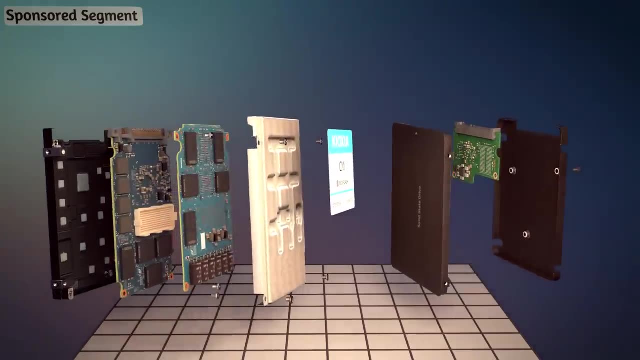 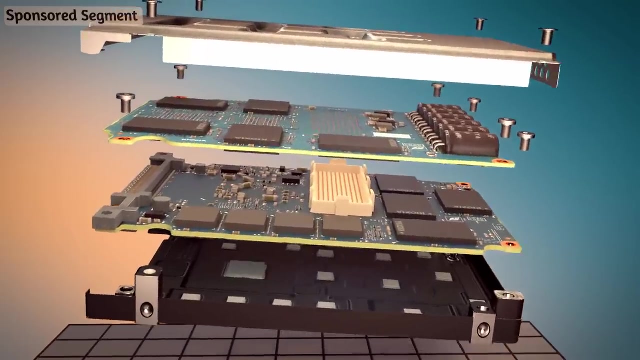 Here's a consumer-class SSD versus this enterprise-class SSD. They look similar from the outside, but are entirely different on the inside. Kioxia provides these leading-quality enterprise-class PCIe NVMe solid-state drives and they can fit in the same space. 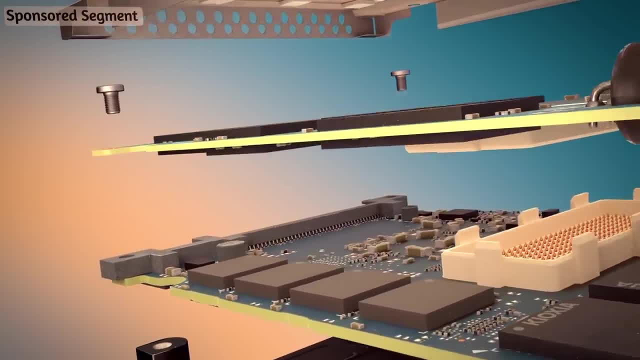 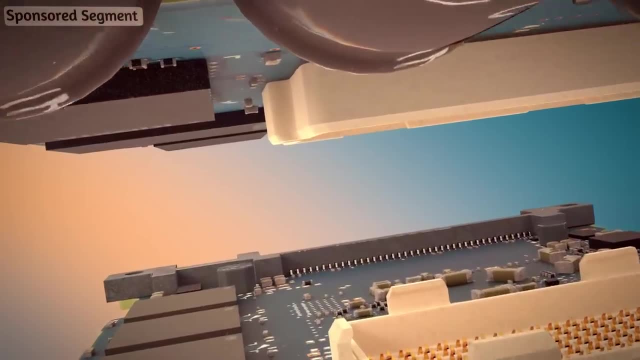 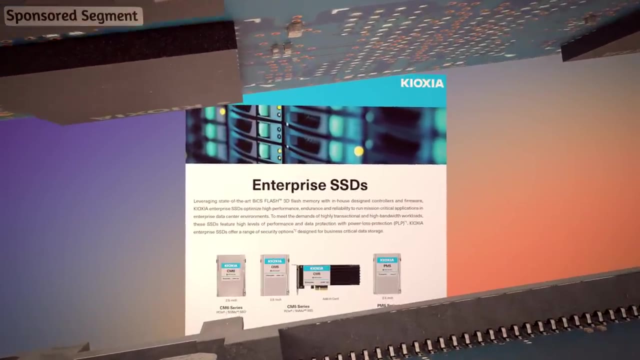 but have capacities up to a whopping 30 terabytes and use a proprietary architecture built with their own controller, firmware and Bix flash 3D TLC memory in order to deliver incredibly high-sustained read-and-write performance and reliability. Check out Kioxia's SSDs. 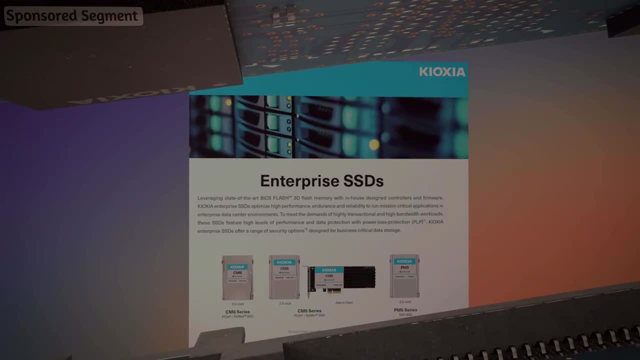 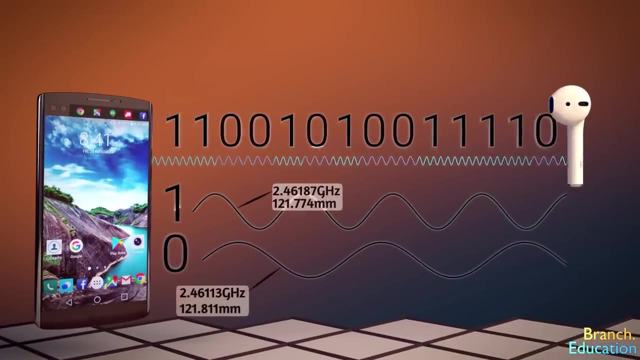 using the link in the description, Let's move on to even more complicated details regarding Bluetooth. The scheme of sending a digital signal or a binary set of ones and zeros by transmitting different frequencies of electromagnetic waves is called frequency shift keying. 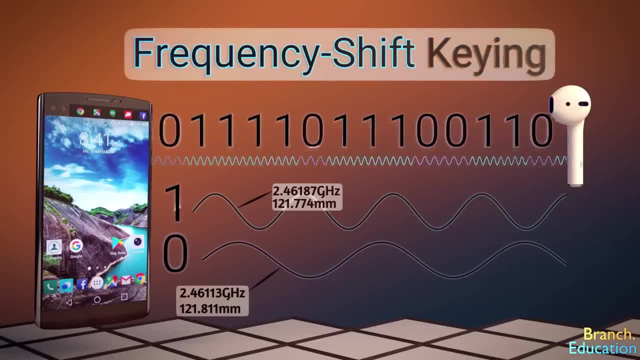 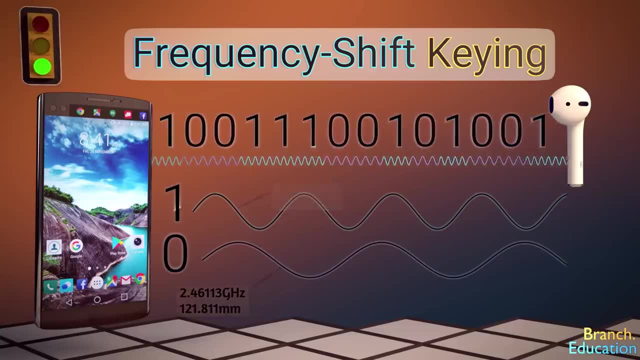 Frequency shifting means that we adjust the frequency, and keying means that a one is assigned to one frequency and a zero to another, just like our traffic light colors. Note that the comparison to a traffic light which emits one color and then another. 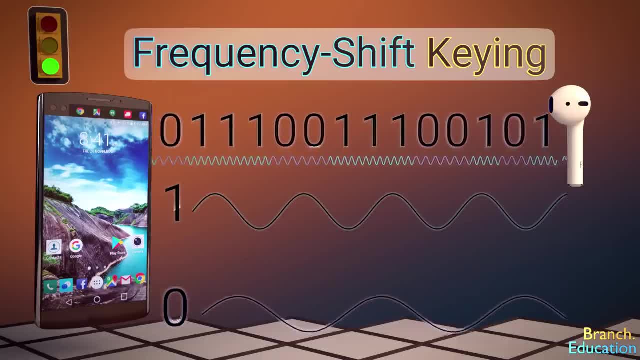 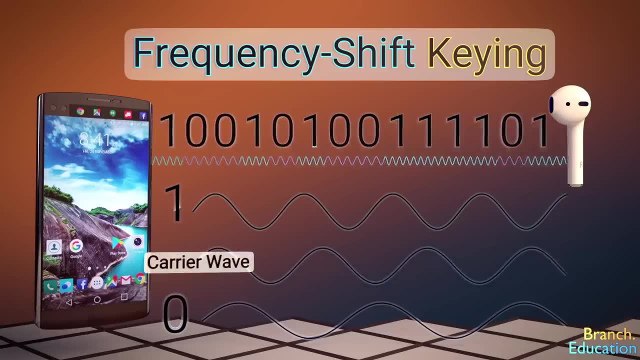 is a little inaccurate, because your smartphone's circuitry generates one frequency called a carrier wave. This circuitry shifts the carrier wave to a higher frequency when it wants to send a one, or to a lower frequency when it wants to send a zero. 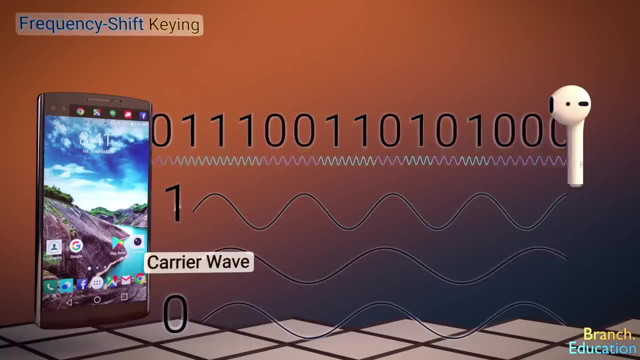 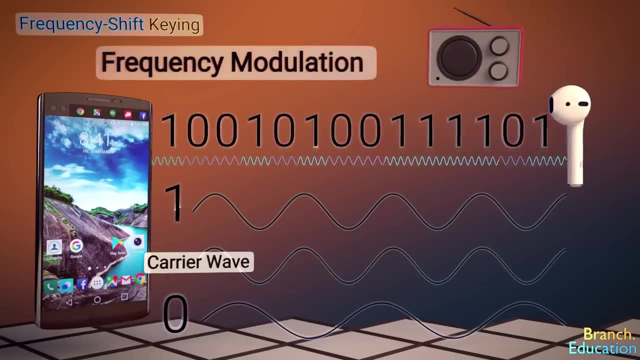 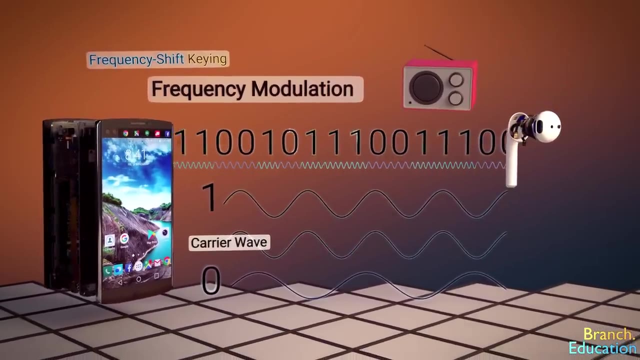 This shifting of frequencies in order to send information is also called frequency modulation, and it's closely related to FM radio. That being said, Bluetooth isn't limited to using just frequency shift keying, but rather it can also use other properties of electromagnetic waves to transmit information. 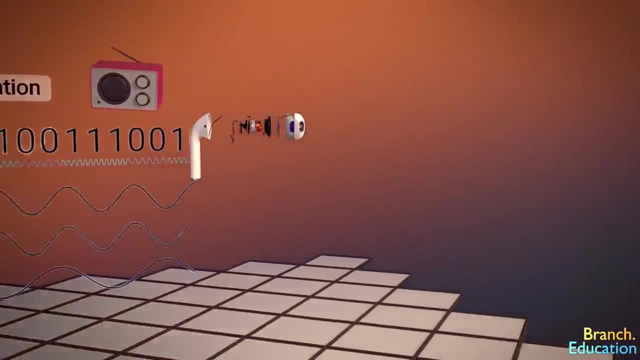 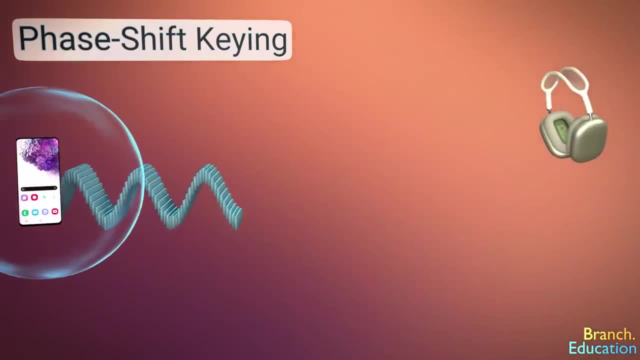 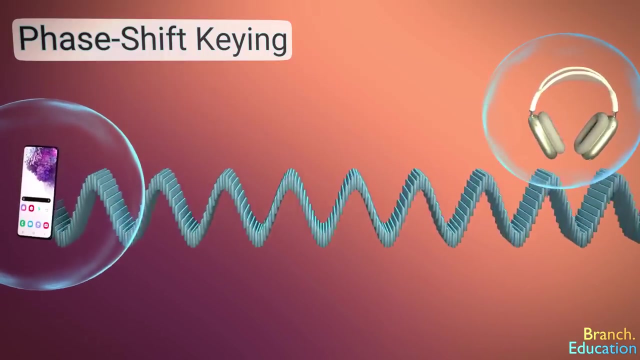 A different method that has higher data transfer rates is called phase shift keying, which is significantly more complicated to explain, but we'll try. An electromagnetic wave's phase is a property that our eyes can't perceive and it shouldn't be confused with the amplitude. 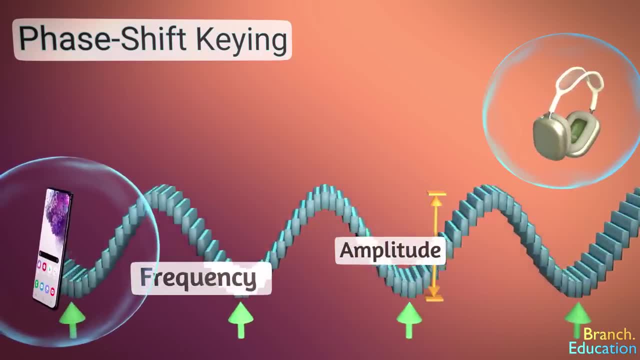 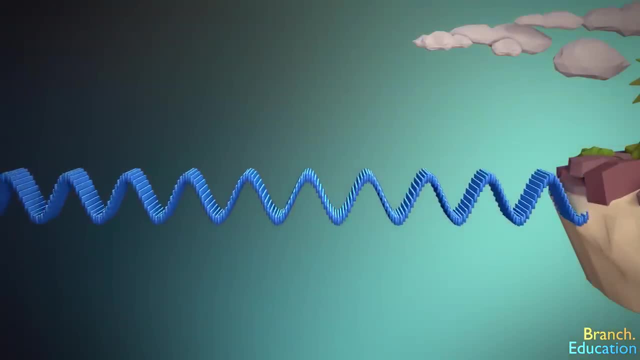 or the frequency or the wavelength. Let's use an analogy: Imagine you're at the beach and you see the waves hitting the shore at a rate of one wave a second. Over a minute you would see 60 wave peaks reach and break on the shoreline. 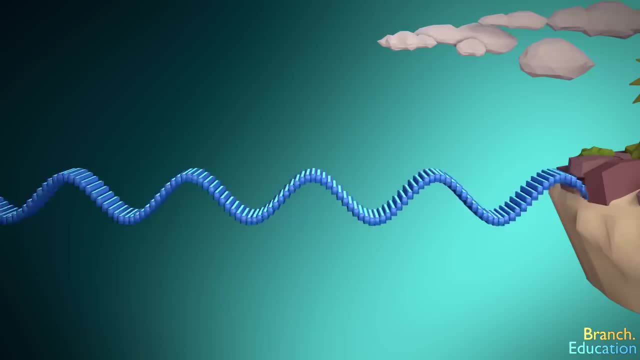 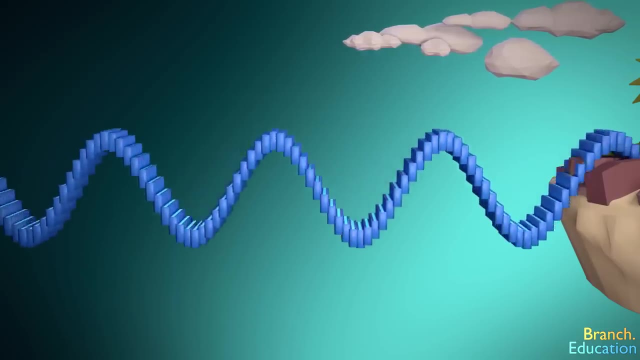 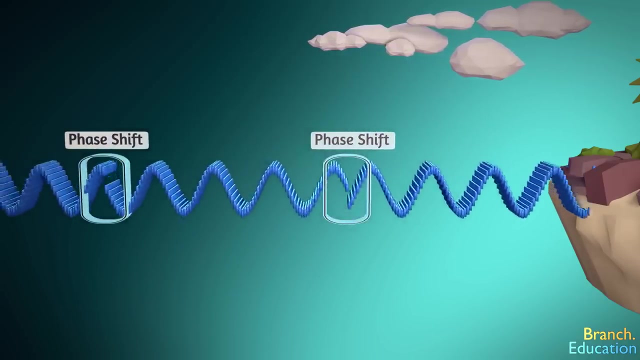 Changing the frequency would be changing how many wave peaks reach the shoreline every second, and changing the amplitude would be changing the height of the peaks and troughs of the waves. However, phase shifting would be seen as breaking up the waves' locations of the peaks and the troughs within a set of wavelengths. 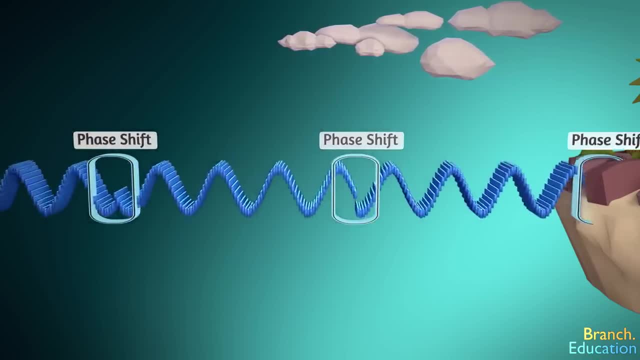 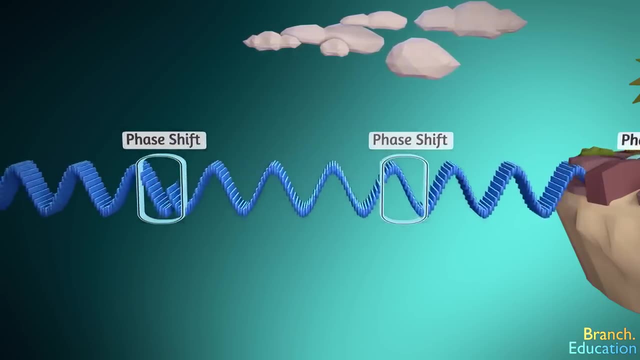 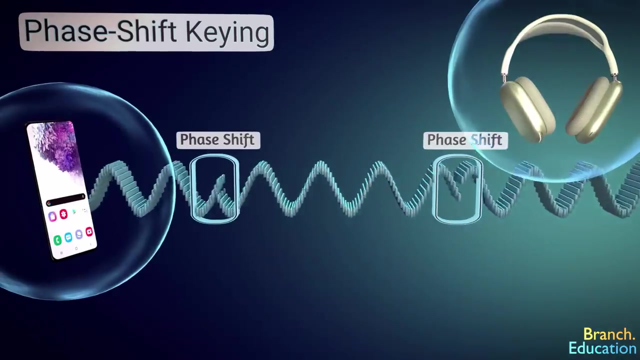 There are still 60 waves over an entire minute, meaning the frequency doesn't change, but as the phase shifts, it's as if the peaks and troughs shift forward or backward within a set of wavelengths. Bluetooth antennas and circuitry in your smartphone and wireless earbuds. 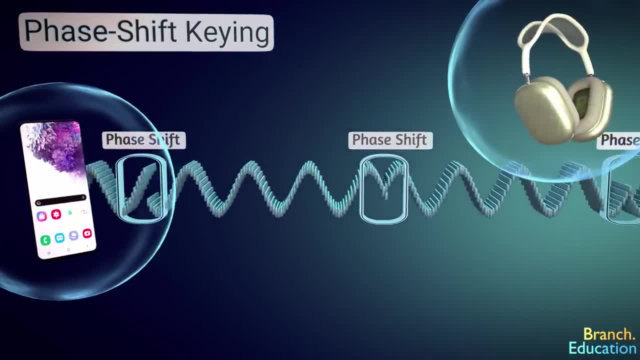 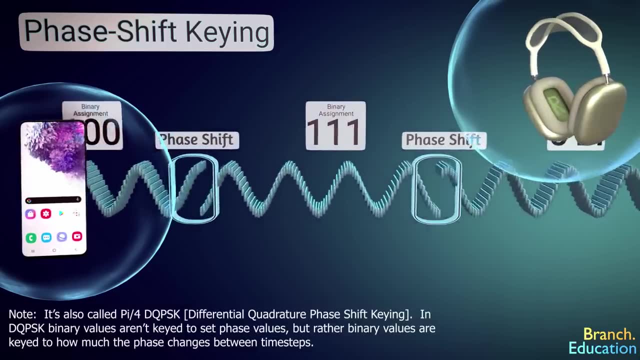 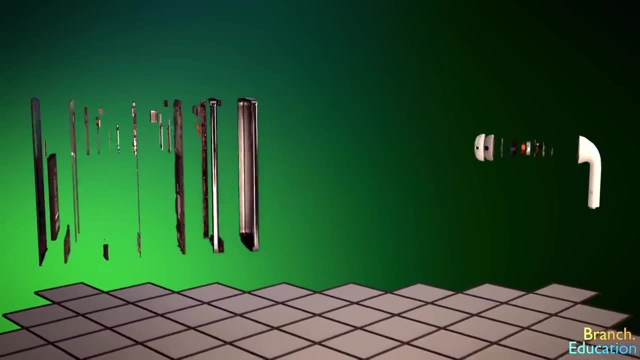 can be designed to emit and detect shifts in the phase of an electromagnetic wave, and binary values can be keyed or assigned to different levels of shifts in the phase of the wave. There are a few things to know, with our examples and explanations. We've talked a lot about your smartphone. 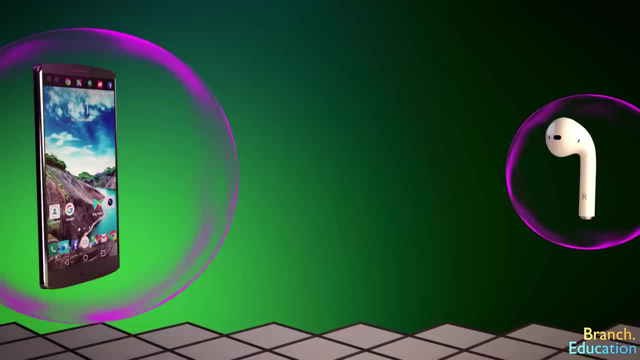 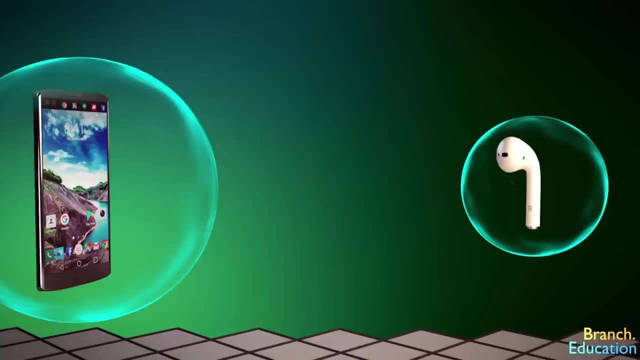 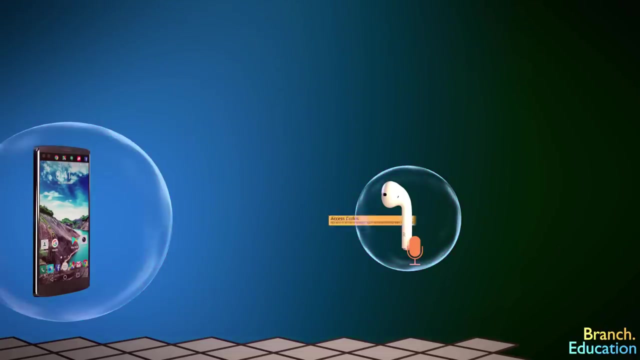 sending information to your wireless earbuds. However, your earbuds also send data to your smartphone. For example, when you're on a phone call using your earbuds, the audio from the microphone in your wireless headphones is obviously sent back to your smartphone. 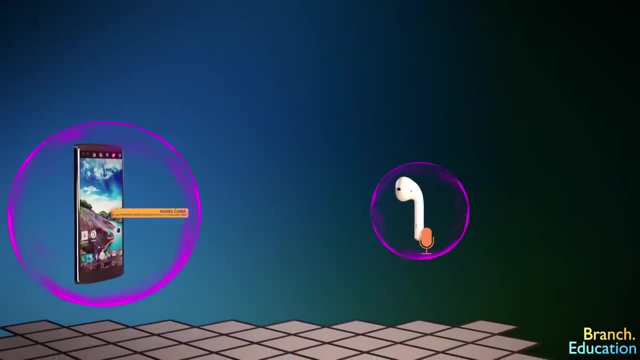 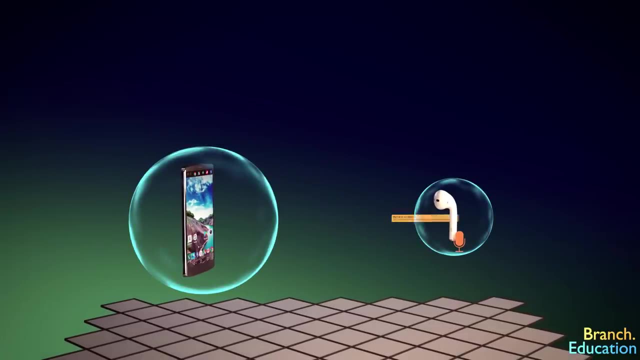 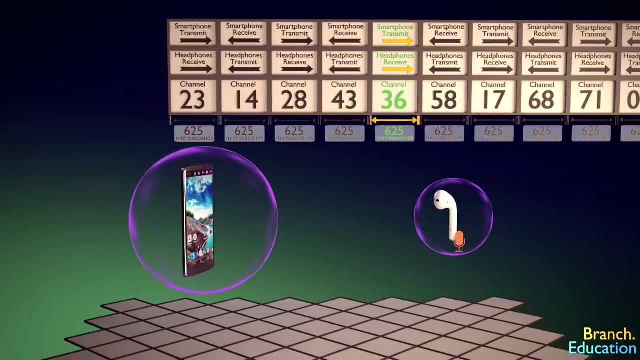 In order for Bluetooth to accommodate this back-and-forth conversation, the smartphone and the headphones alternate transmitting and receiving data while maintaining the frequency hopping schedule. During one 625-microsecond time slot, your smartphone will send one packet of data to your headphones along one channel. 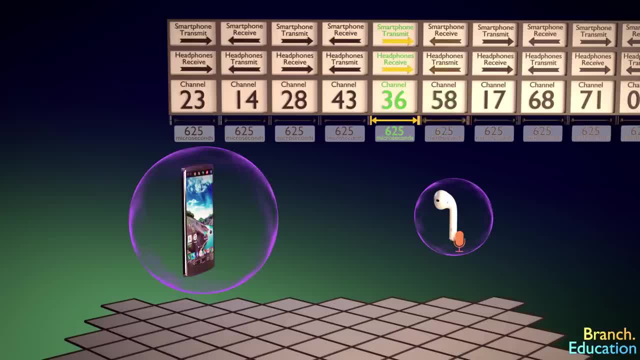 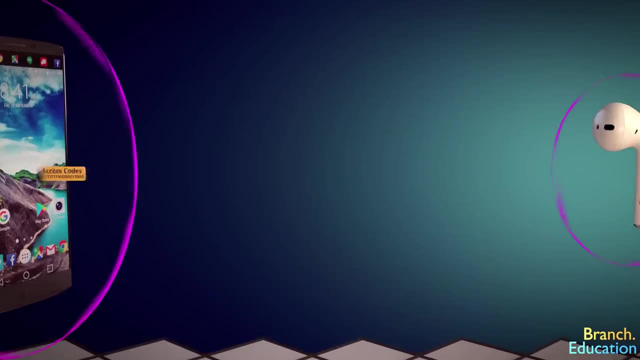 and then, during the next 625-microsecond time slot, your headphones will send one packet of data to your smartphone along the next channel in the frequency hopping schedule. Also, as we mentioned earlier, a Bluetooth packet is composed of three sections: access codes of 72 bits. 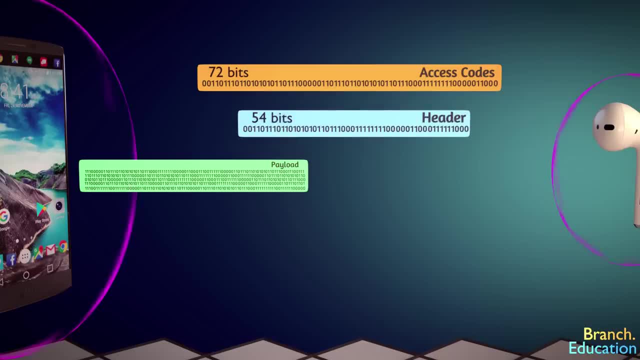 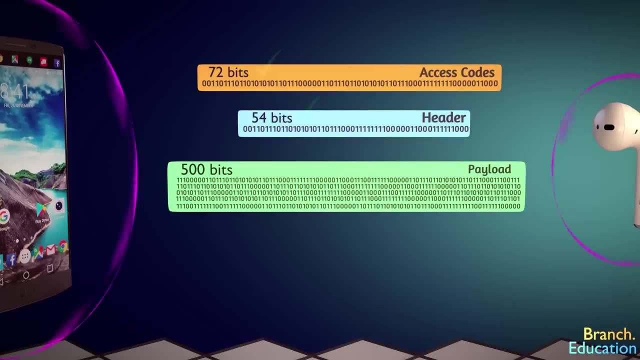 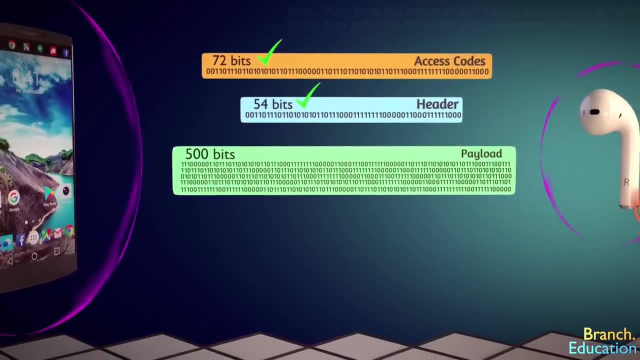 a header of 54 bits and, for example, a payload of 500 bits. The number of bits in the access codes and header are pretty close to those mentioned. However, the size of the payload which is specified using the header can vary widely, between 136 bits. 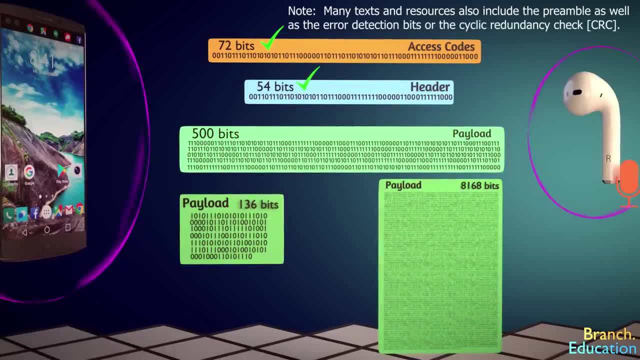 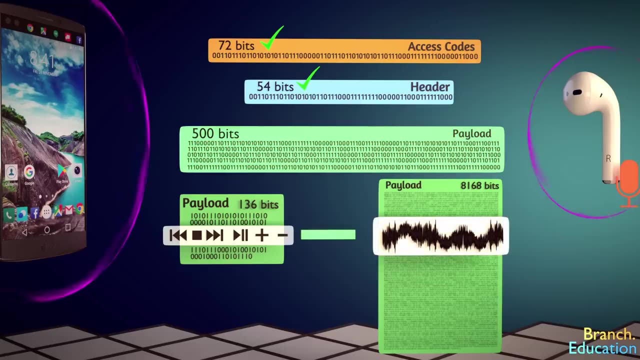 and 8,168 bits, depending on the requirements of the data being sent. For example, simple commands from your headphones like pause or play the music would require far fewer bits than sending or receiving high-quality audio. An additional caveat is that 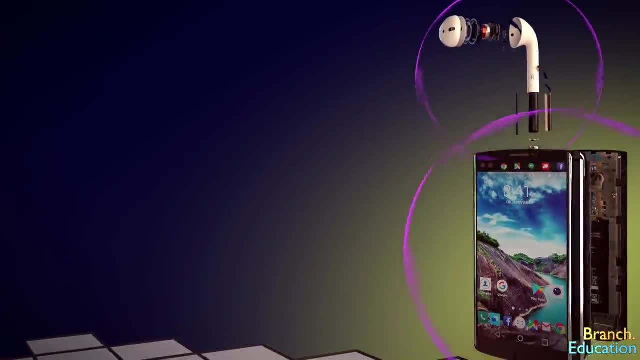 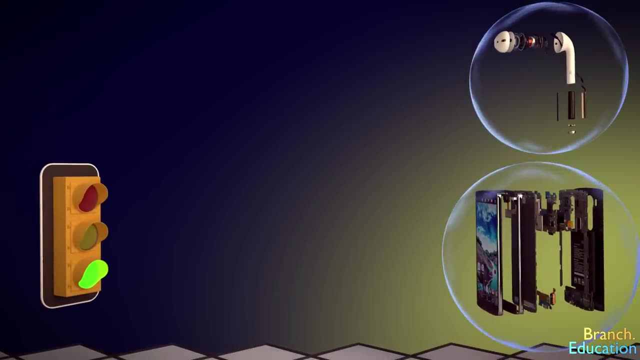 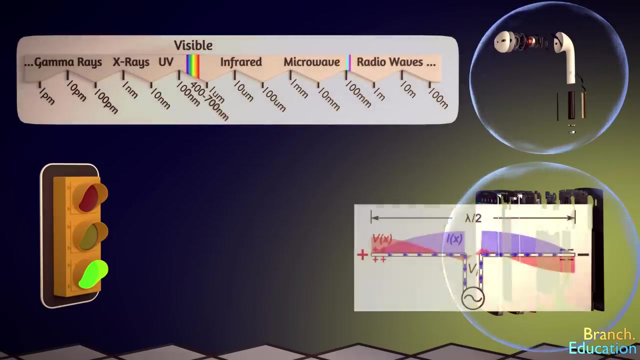 the electromagnetic waves sent and received from the antenna in your smartphone and earbuds and the light from a traffic light share the aspect that they both function within the electromagnetic spectrum. However, the principles that govern how your smartphone and headphones generate and receive those electromagnetic waves